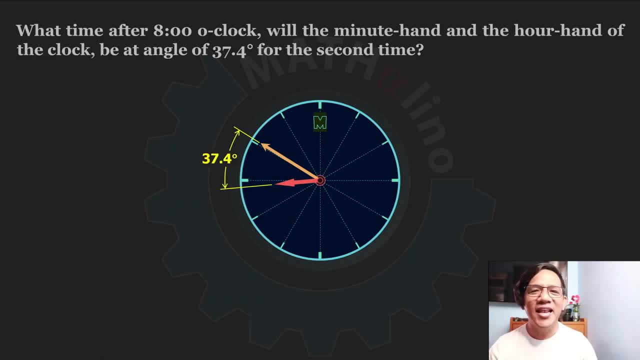 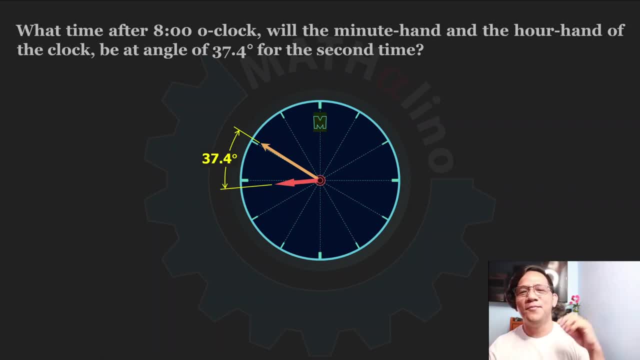 5 seconds. starts now 1,, 2,, 3,, 4, 5.. Are you done? If you still need time, just pause this video and continue later watching, if you're done. solving this problem. solving the problem. to solve this problem, excuse me, to solve this problem, uh, swiftly. 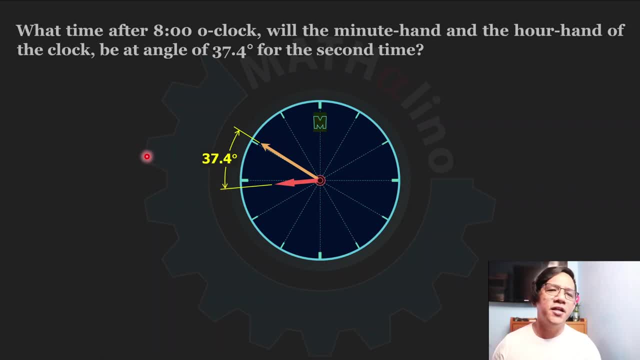 we are going to use two strategies. number one is by multiplying, is by using 60 over 11, and the other one is by using 2 over 11.. okay, you may wonder what are these numbers? just continue watching. uh, this 60 over 11. we are going to multiply this by the hour mark. okay, and our 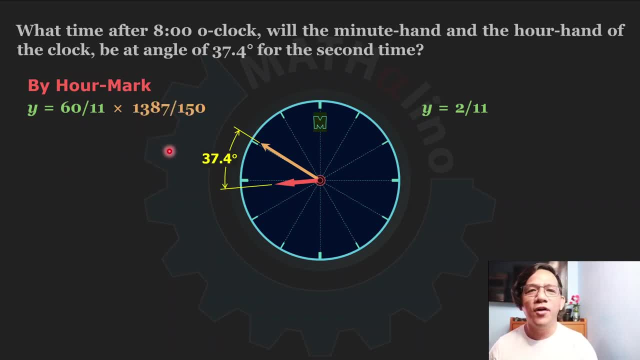 marker is 1387, all over 150.. we will get uh for it for this sec, for this: 2 over 11. we are going to multiply this by the angle, and the angle here is actually 277.4. all right, regardless of which one you are going to use, you will come up to the same answer, and that is 50.44 minutes. 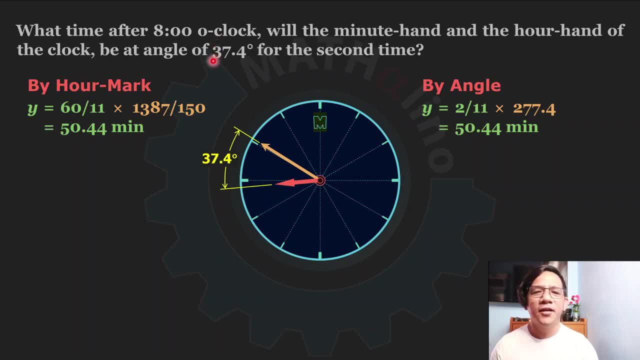 which means that the time after eight o'clock where the hour hand and the minute hand subtend an angle of 37.4 degrees from each other, from each other for the second time, is 8: 50.44. that's the answer, very precise, up to the hand attempts or hundred. 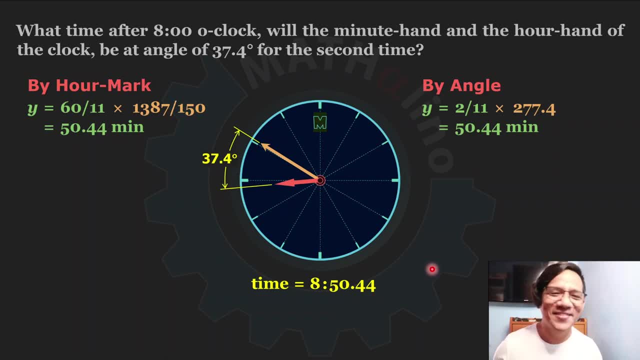 hundreds, digit and minute. all right, you may wonder what? where these numbers came from, what? what is that? 60 over 11, 2 over 11? where this came from? 1387 over 150. you have so many questions in mind. that's why continue watching this video until the end, because my goal here is for you to use this. 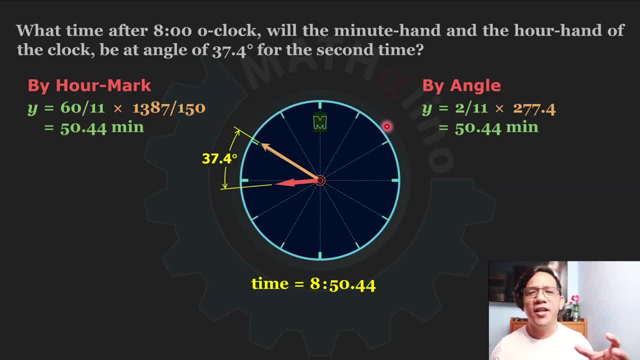 use this uh approach with utmost confidence. we're not going to compromise the the principles behind the clock problem. okay, in fact, i hope this will open a door for you so that you can develop your own strategy in creating uh solutions like this, which is uh, what, what? what we call this shortcut solutions. all right, i hope you can develop your own shortcut. 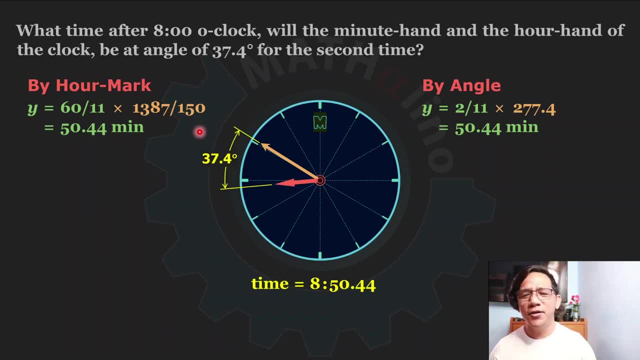 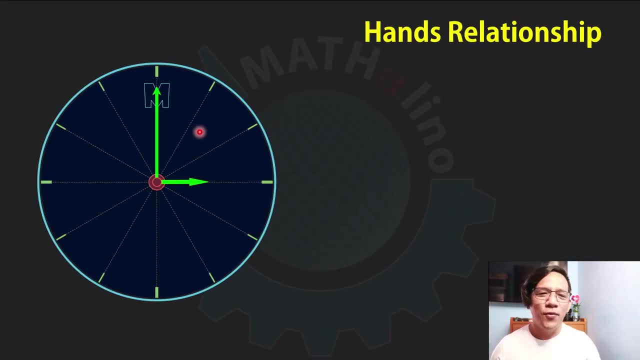 solution. okay, let us discuss the principle. let's go back to the very basic: the relationship between the hands of the clock. we have this three o'clock- uh sharp- the minute hand and the hour hand. okay, then let us call that the distance between the hour marks the 12 o'clock. 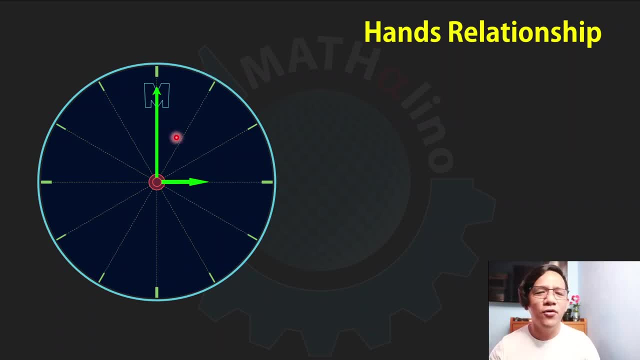 mark and the one o'clock mark, one space. okay, we know that if the minute hand will rotate a total of 360 degrees, that is actually one hour, which means that this, this, our hand, will go from three o'clock mark to four o'clock mark and if we call the distance between the hour marks space, this: 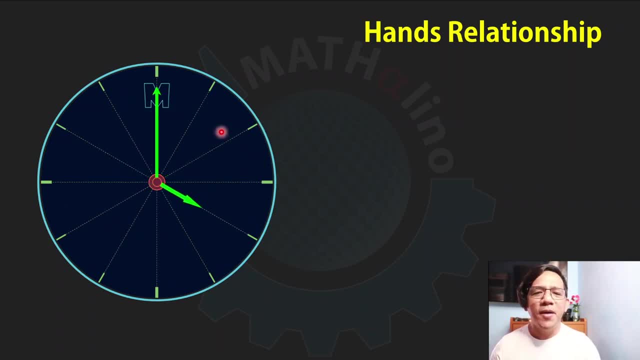 minute hand will rotate 12 spaces. we have one, two, three, four, five, blah, blah, blah, blah- 12 spaces, while the hour hand, that is the movement of the minute hand, while the hour hand rotate from three o'clock mark to four o'clock mark. that is only one space and this is the relationship between the 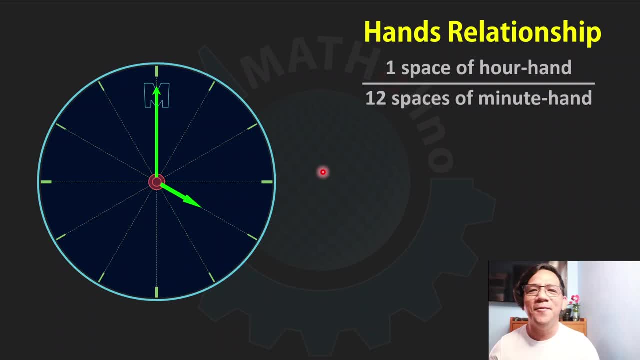 hour hand, the movement of the hour hand and the minute hand. okay, what is the meaning of this cushion one over twelve? it means that every movement of the minute hand, the hour hand will respond one over twelve of that movement. okay, the hour hand will also move one over 12 of the. 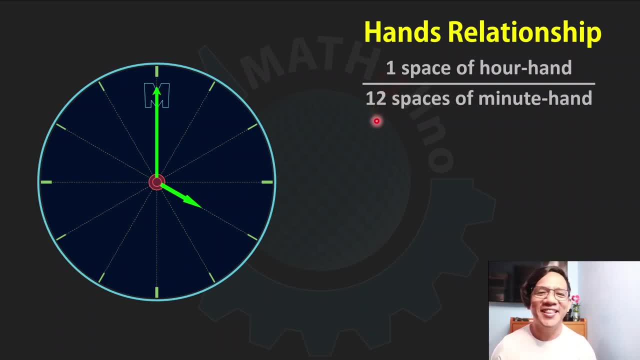 movement of that minute hand. can you see that? let us say: let's go back to three o'clock mark three o'clock sharp. let us say that, uh, the minute hand will rotate y minutes. okay, let us say: the y minutes is here, that's it. that is the y minute measured from the 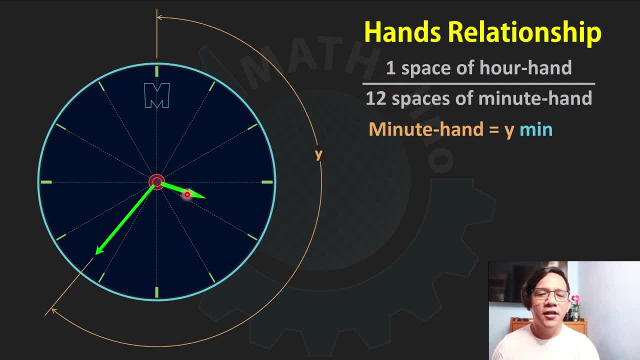 12 o'clock mark. okay, of course the hour hand will also rotate, but it's not uh. it will not uh go to 4 o'clock yet because it's not yet one hour. so this is the movement of the hour hand. the question is, how much is this movement? we can express this in terms of the movement of the. 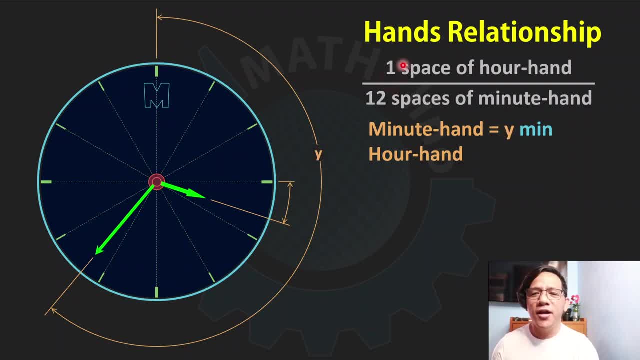 minute hand and the movement of the minute hand is why, according to our relationship, this movement is one, one over twelve. of this movement, take note our unit. also, for this movement, the movement of the minute hand takes 6 minutes. you get that. that's it, most of the board exam. 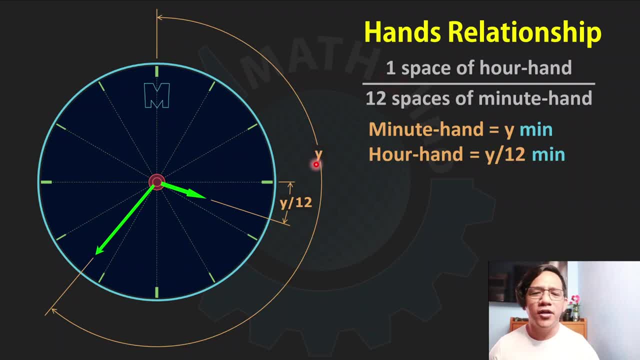 in. uh, most of the problems in the board exam are only up to this point, where we are going to do to use the relationship between the minute hand and our hand, but of course, for uh discussion purposes, we are going to include in our discussion the movement of the second hand. if you have a, 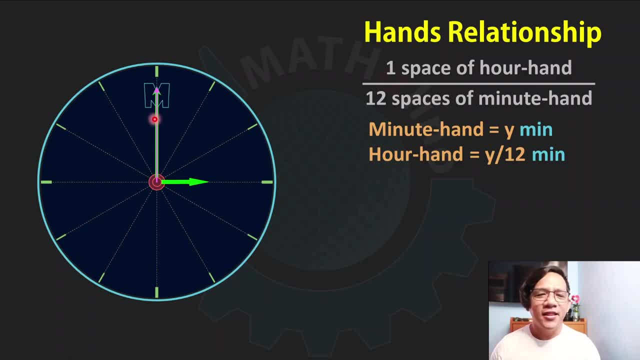 secondhand. okay, that's the second hand. let us say that this, uh, let us say that, that this standardined, that the distance between the, the small marks here for the second marks: okay, one minute marks one minute. one minute, one minute, a total of five minutes here. okay, also a space. or let us say that: 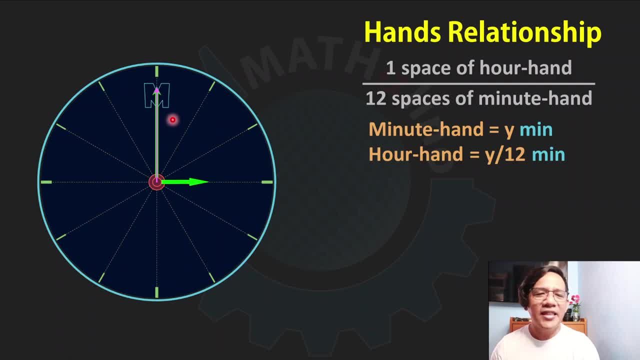 if the, if the second hand will rotate, will create 60 seconds. okay, the minute hand actually move one one space. that is the relationship. okay, let us do that. i think i need to remove my video feed. okay, let me check if i have removed the media feed, video feed. all right, let's continue. 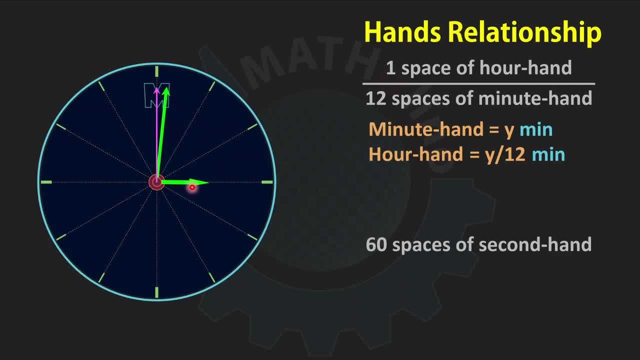 we have this. let us repeat: actually the our hand also moves very, very small amount. you can see that if you are going to reverse the process, observe this, our hand, the movement of this, our hand. one, two, three, four, what's that? that is the movement of the our hand. okay, very small movement. now let's go back to our original. 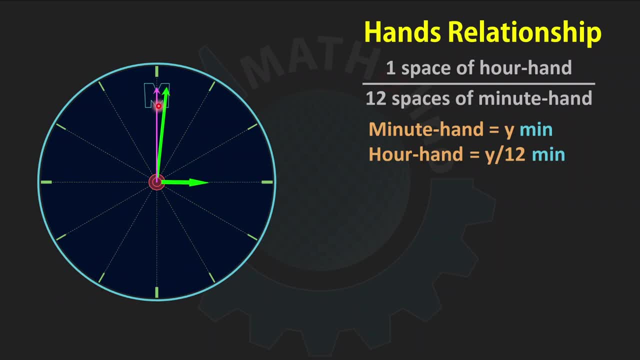 position. we have this: uh movement of the second hand is 60 spaces- okay. the second hand moves 60 spaces. the minute hand is 60 spaces- okay. the second hand moves 60 spaces- okay. the minute hand moves one space- okay. this is the relationship, the meaning of this, every movement of the second hand. 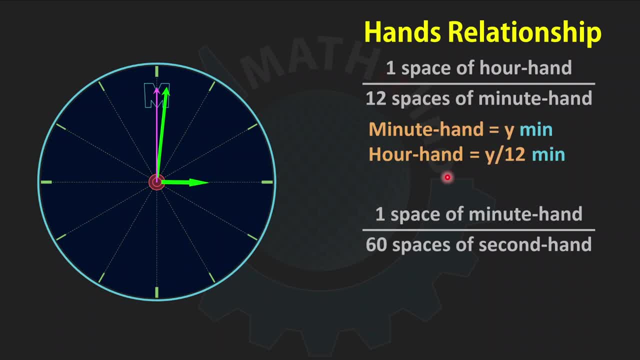 the like, like the relationship in the minute and our hand. every movement of the second hand, the minute hand will move 1 over 60 of that movement. let us say that our second hand moved by y seconds. okay, of course, according to this relationship, the minute hand also moved by y over 60. according to: 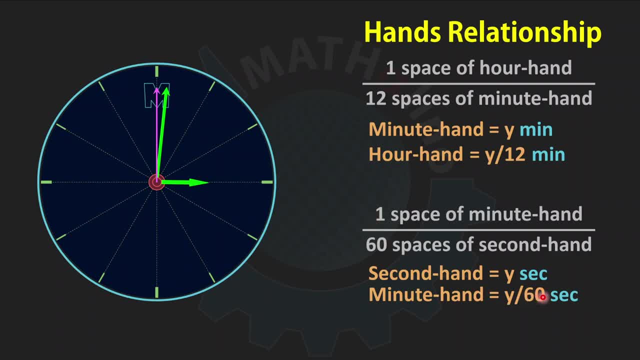 this relationship: y over 60.. and take note: our unit now is second. because the lowest, lowest unit of time is second, we are going to use the lowest unit of time. how about the our hand? what is the movement of the our hand in relation to the movement of the second hand? 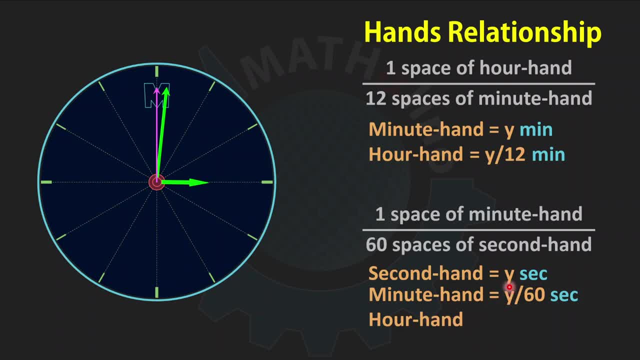 first, the move, the, the our hand will move 1 over 12 of this movement of the minute hand. 1 over 12 times 1 over 60, that will become 1 over 720 of the movement of the second hand. okay, seconds also. that's it. that's the underlying principle. and you couple that with the geometry. 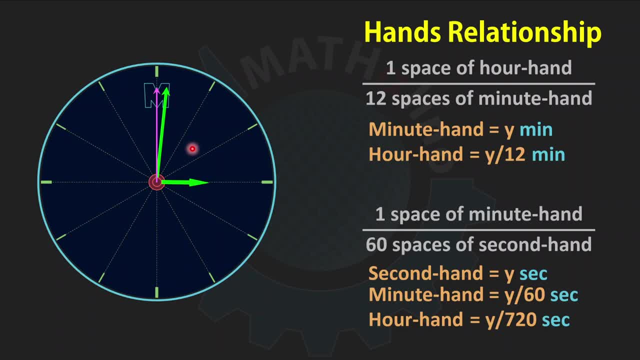 boom, chicken joy. that's the relationship between the movement of the hour hand and the second hand. you can also do angle, because this is 60 degree, I know, this is 30 degrees- okay, 30 all over, uh, one space actually is 30 degrees here. and and all over 360 degrees- okay, the same one over 12.. you can also 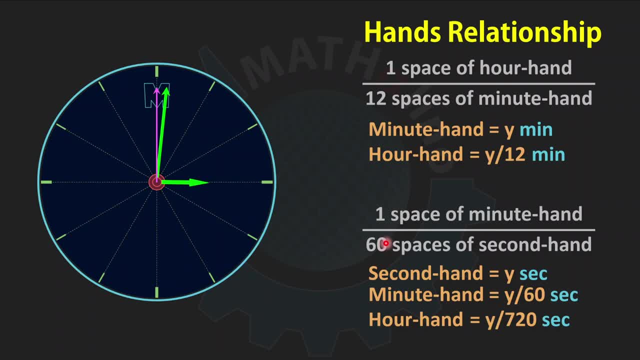 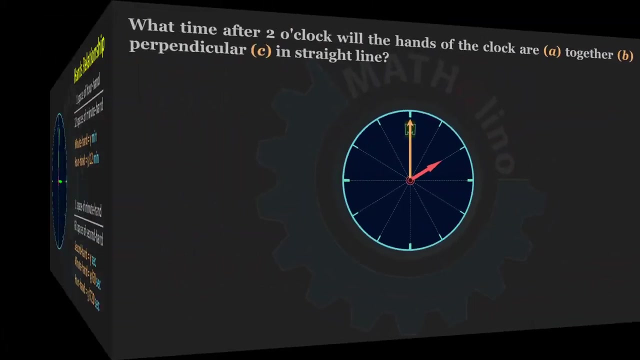 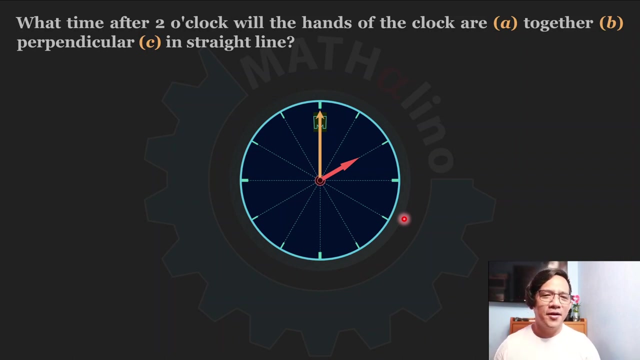 use here: uh, 1 over 60.. very, very easy, 1 over 1 over 60.. one minute, this one movement of the second hand, one space between the marks here. all right, let us use this relationship with examples. okay, example: what time after two o'clock will? the hands of the clock are together, perpendicular, in a straight line for. 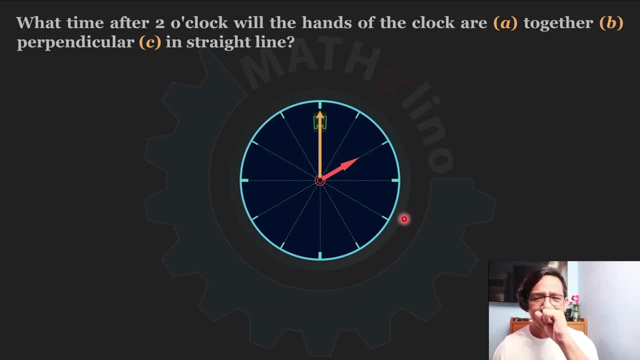 the first time probably. these problems, this type of angle relationship or the distance between the hour hand and the minute hand, are very common in clock problem. most of the high school materials are, with this statement, together for the first time, perpendicular for the first time, perpendicular for the second time, in a straight line for their first time, and so on. okay, so what time after two. 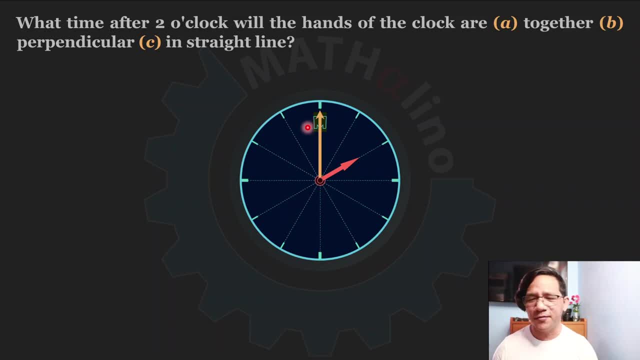 o'clock. let us discuss this by principle based discussion. okay, according to what we discussed previously, that relationship of the minute hand and our hand, so let us move this minute hand. okay, now this is the position of the, of the hands of the clock when they are together. 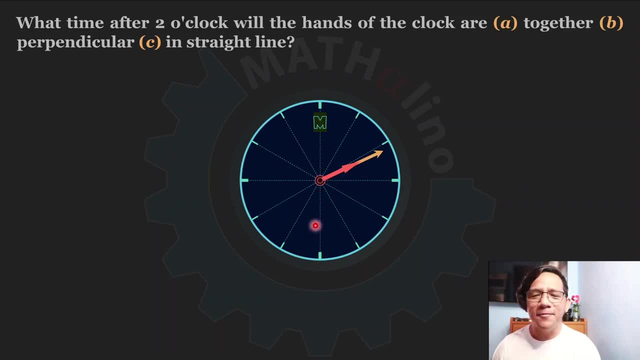 the question is: what time is it? how many minutes? it will happen after two o'clock. let us call that number of minutes y, so let us solve for y. it will happen at two y. okay, two, the time is two y, of course, from the two o'clock mark up to this final position. 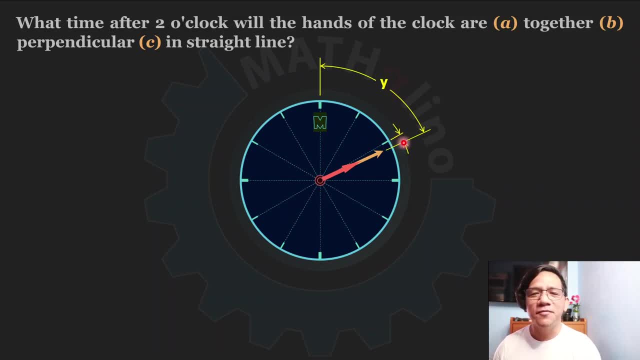 the hour hand move also this much. this is small increments, this is small amount. what is this movement? by principle, this is equal to y over 12 of the movement of that minute hand. that is why, over 12. how to find that hand? to find the y based on the figure. very easy, we have this. y is equal to what? 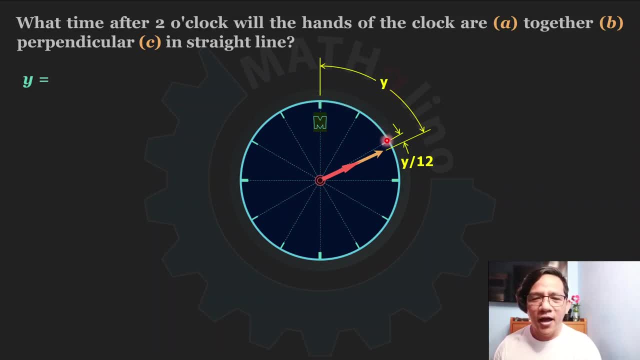 from the 12 o'clock now mark up to the 2 o'clock number: how many minutes we know that we are going going to discuss. we are going to use the the equation in minutes. we are going to write the equation in minutes: minutes of time. number of minutes of time. we have this one, five, ten minutes. 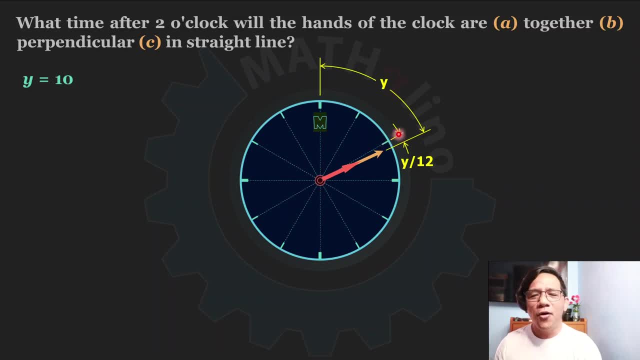 this mark. okay, ten minutes plus y over 12. to get into that position of the y plus y over 12, solve for y. we have 1 minus 1 over 12. that will become 11 over 12 of y is equal to 10. 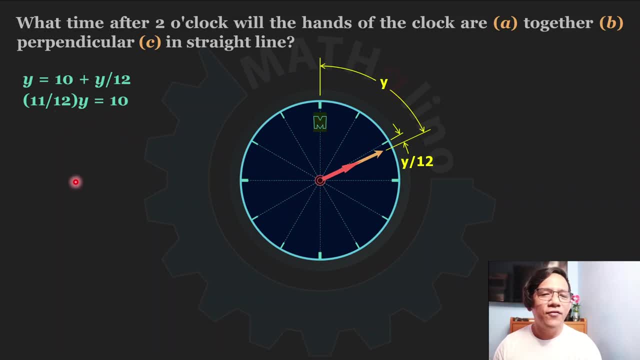 okay, 10 divided by 11 over 12, that will become 120, all over 11 minutes. right then, the time, of course, which is the required is equal to 2: 1 over 20 over 11 is actually 10.91, 210, almost 211. 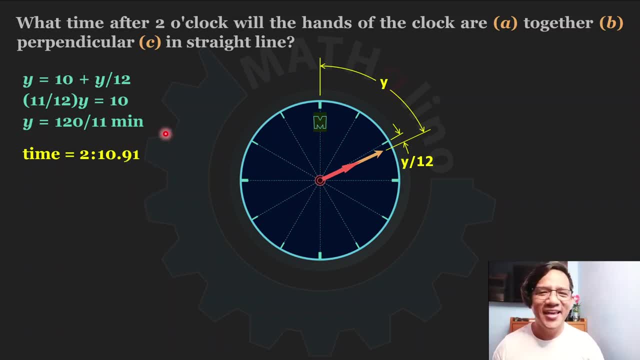 okay, that is the answer. okay, how about letter b- perpendicular- perpendicular? okay, how about letter b- perpendicular? okay, how about letter b- perpendicular- they are perpendicular. let's move to perpendicular position. that's it. they are perpendicular for the first time. okay, what is this time? let us call this again 2y. that is the value of that is the why we are going to solve this. 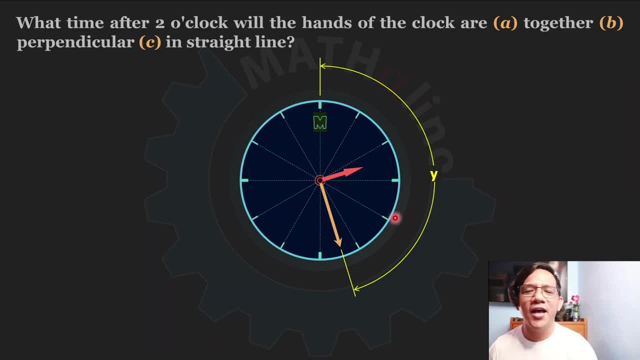 distance. okay, movement of the minute hand again from the 2 o'clock mark to the final position of the hour hand. this distance is equal to what y over 12, that is, y over 12. so what is the value of y? let us write the equation from the figure: y is equal to this position or this mark, two o'clock. 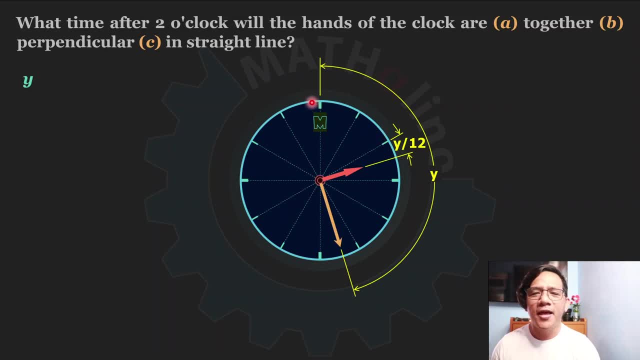 how many minutes from the 12 o'clock mark? that is 5- 10. that is 10 minutes plus y over 12 10 minutes. we are going to find the distance from this point up to this point okay, that is 10 plus y over 12. 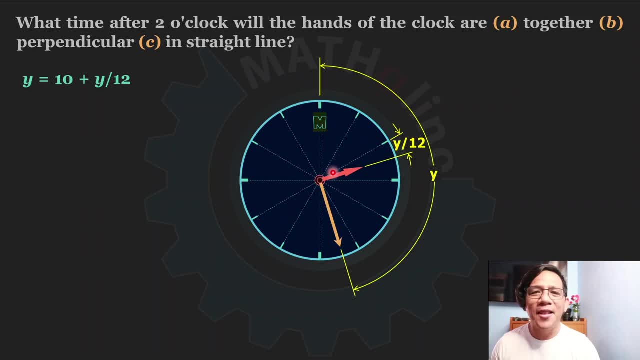 all right, plus how many minutes. right angle, 90 degrees of 90 degrees is how many minutes of time? not minutes of angle, how many minutes of time? that is actually 15 minutes, right, that is 3 uh 12 o'clock, 12 o'clock mark and 3 o'clock mark. that is 15 minutes. they are right at right angle also this one. 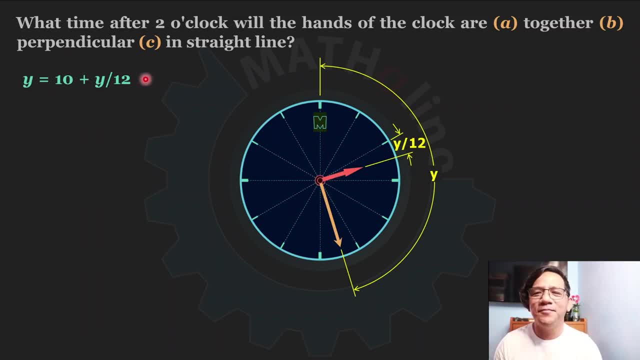 they are at right angle, perpendicular to each other. okay, so 15 minutes plus 15. i will repeat: we have this: 10 plus y over 12 plus 15 minutes. solve for y. we have 1 minus 1 over 12. 11 over 12, that is equal to 25. okay, 25 divided by 11 over 12, that is 15 minutes plus 15 minutes. 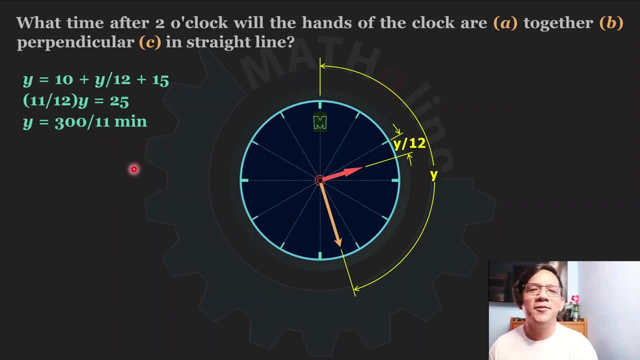 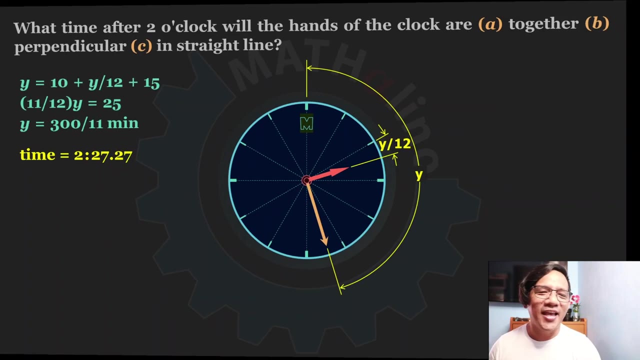 we get this 300 over 11 minutes. the answer is 2, 3. 300 over 11 is actually 27.27. okay, that is the answer right next in a straight line, in a straight line. so when we say in a straight line there, because 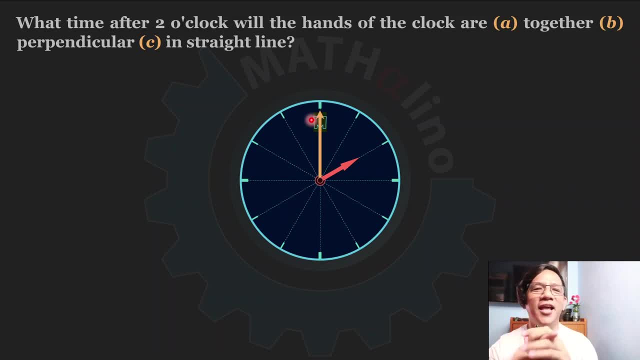 when they are together, they are also in a straight line, but when we say in a straight line, they are pointing in opposite directions. okay, so meaning the position of the minute hand and the hour hand is this one, it's this one. okay, where's my laser pointer? what time is it we have this? let us call this number of minutes. 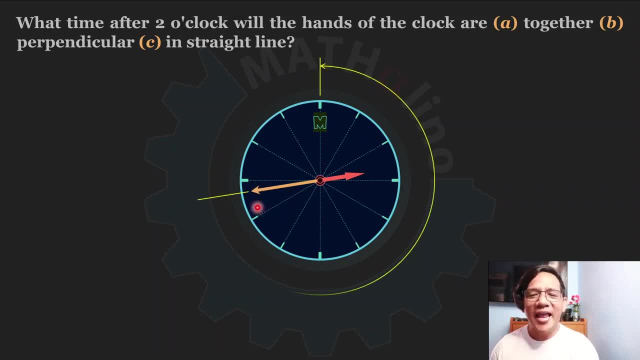 made by by the minute hand, again y minutes. and of course the hour hand from the two o'clock mark moves 1 over 12 of this movement. that will become y over 12. okay, what is the value of y from the figure? again, y is equal to. this is again 10 minutes, okay, plus y over 12 again. 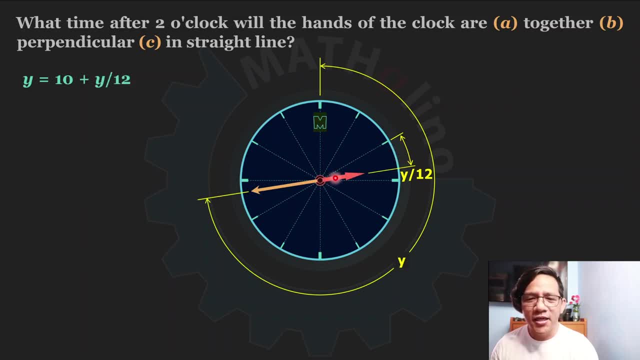 y over 12. but now- but this distance is straight line- is 180 degrees. 180 degrees in minutes of time is actually 30 minutes. okay, it's like 12 o'clock and the six o'clock mark that is 30 minutes. okay, we have this. 1 minus 1 over 12 is 11 over 12 is equal to 40. all right, what is the value of y? 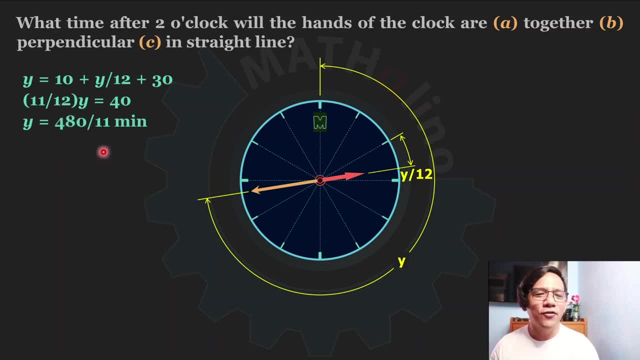 40 divided by 11 over 12, that is equal to 480 over 11. and this is our answer: 243.64. all right, that's the basic solution, but the purpose of this problem is the shortcut of this video. is the shortcut. let us solve this problem by our 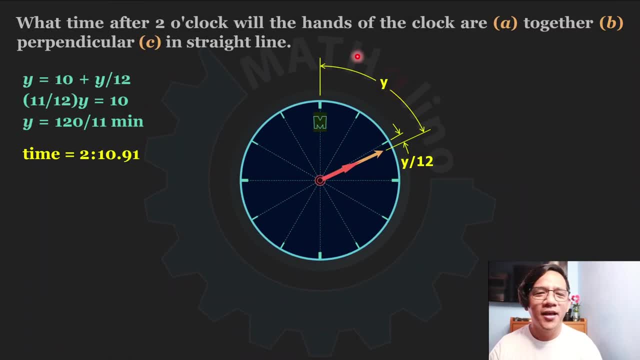 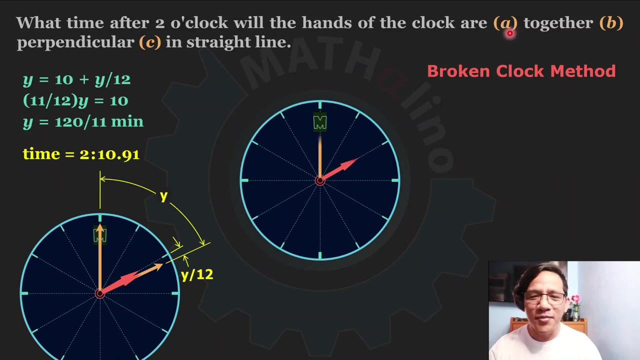 shortcut method. actually, this shortcut method, I call this the broken- okay, the broken- clock method. let us do the broken clock method. let us start with letter a together for the first time- this is the two o'clock mark- and let us rotate this hands of the clock so that they will be 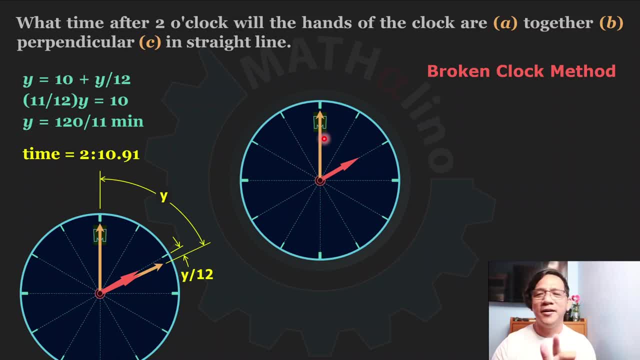 in: uh, they will be together. okay, they will be in this position. sir, something is wrong. the move the hour hand did that move? you got it because this clock is broken, that the hour hand is stuck at that position. only the minute hand will move. okay, now for the solution using using the hour. 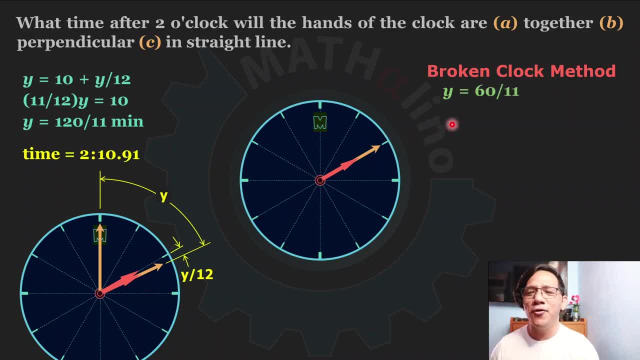 marks. we are going to use the number 60 over 11.. you can memorize that number, okay, sir. where is that where that number came from? we are going to discuss that later on this video. 60 over 11.. times, what times? the hour marks where the, where this uh minute hand is pointing this this hour, the, the. 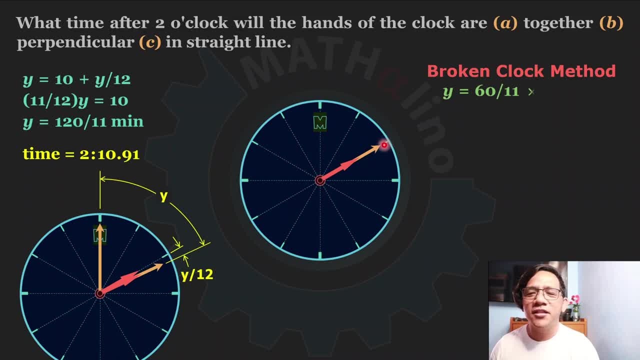 hour mark. the minute hand is pointing at two o'clock mark. so this is times two and that is the answer: 120 over 11.. okay, or you can also use the angle. you can also use the angle. take note that the hour mark is measured from that, from the 12 o'clock. 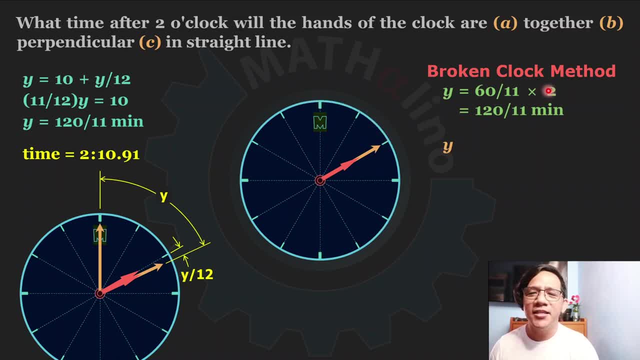 mark to the final position of the minute hand. that is the uh the hour marks. for the angle, we are going to use 2 over 11.. and to measure the angle, it came from the 12 o'clock mark to the final position of the minute hand also. okay, the same measurement, only that. 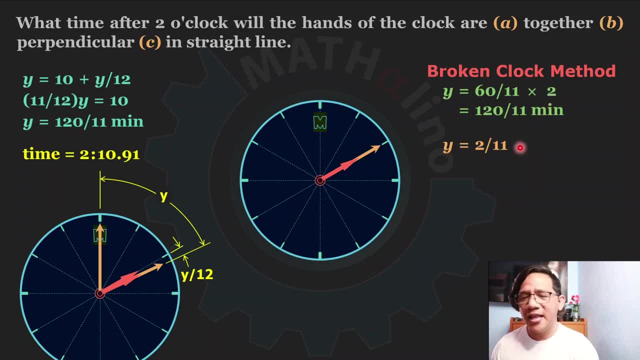 this one is the hour mark and here is the angle. this is 60 degrees. okay, from 12 o'clock mark to the final position of the minute hand: 60.. and that is the answer: 120 over 11.. okay, it's up to you which one you are going to use. you may use this one or you may use this one, doesn't matter. 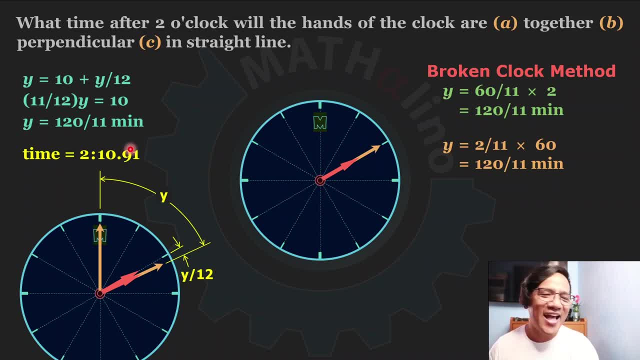 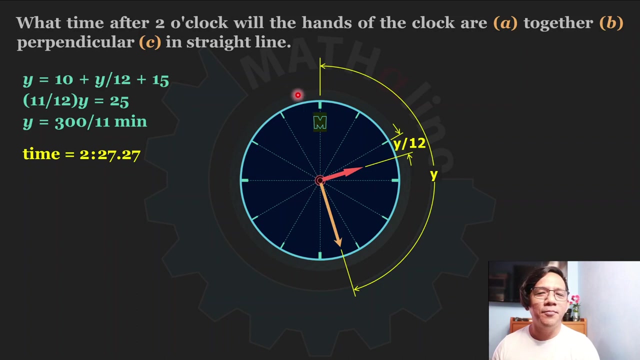 okay, that's the answer, baby. how about perpendicular? for the first time, I think you can do that in less than five seconds, less than one second. if you have a fast hand in calculator, you can do this in in one second. how about this letter b perpendicular? so let's go back to our for uh solution in the previous. 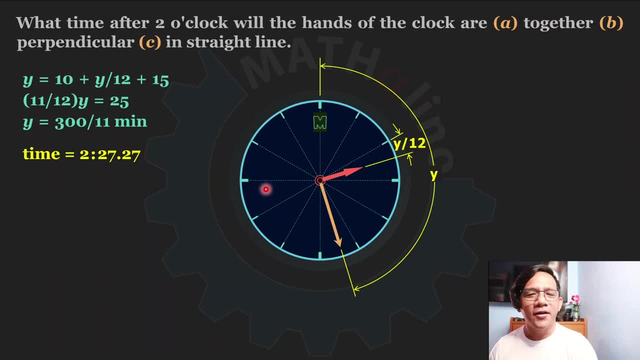 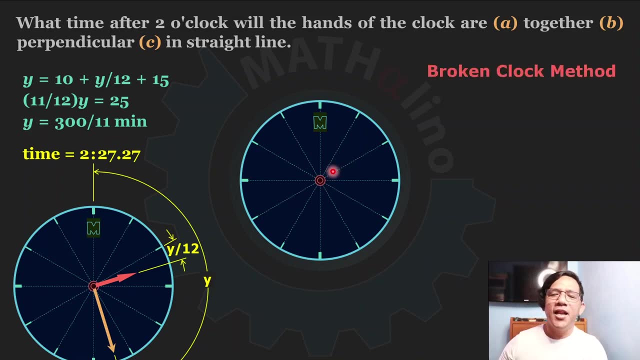 concept-wise, concept-based solution. okay, let us remove this figure first and let us initiate at 2 pm, initialize at two, two o'clock. i mean using the broken clock method. let us move this minute hand and the the hour hand will not move because this clock is broken. 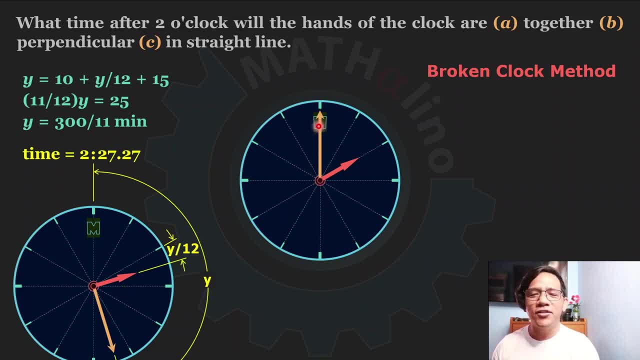 okay, and let us position this minute hand so that it will become 90 degrees to this hour hand. that is perpendicular. they are perpendicular meaning this minute hand will go in this at this point. the five o'clock mark, this is 30, 60, 90. they are perpendicular to each other. 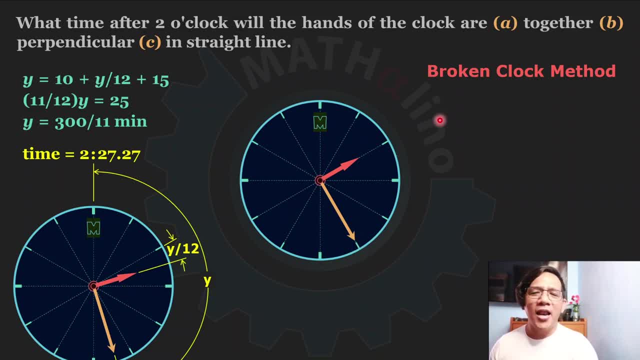 by our clock by by by our mark method, the broken clock method, using the hour mark, that will be 60 over 11 times 5. okay, that is the answer. 60 times 5 is 300. all right, by using the angle, the angle from, we will use 2 of 2 over 11 times the angle from 12 o'clock mark to this point, the 5 o'clock mark. 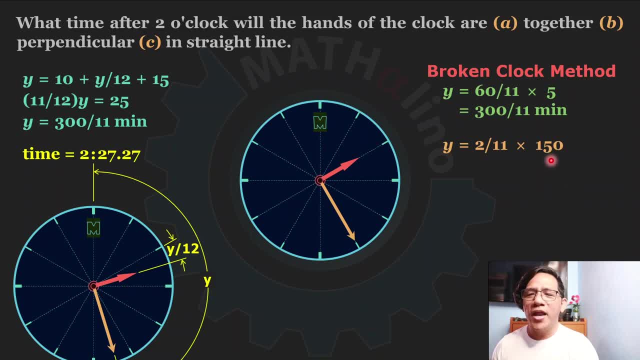 that is 30 times 5. okay, that is 150. i know, not 30, that's correct. 30, 30, 30, 30 times 5. 1, 2, 3, 4, 5. 30 times 5, that is 150. okay. 150 times 2: the same answer: 300. all over 11 minutes. 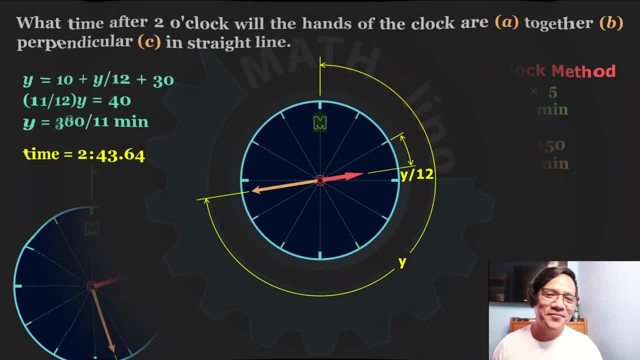 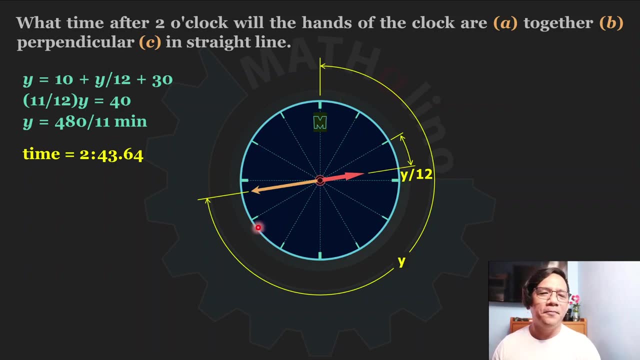 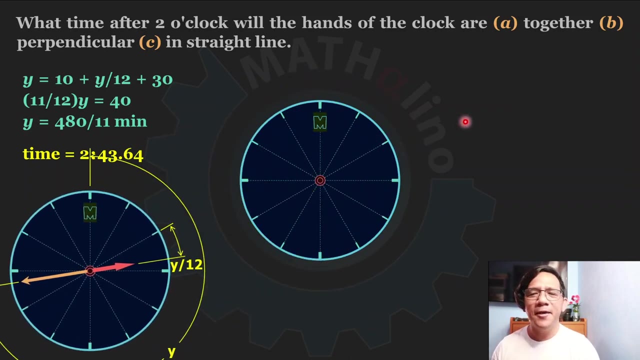 very easy. how about a straight line? okay, how about in a straight line? uh, this is the, this is our solution. or a figure from from: uh, concept based method? okay, let's move that. and by uh, broken clock method, we're not going to, we're not going to draw, i'm going to draw the. 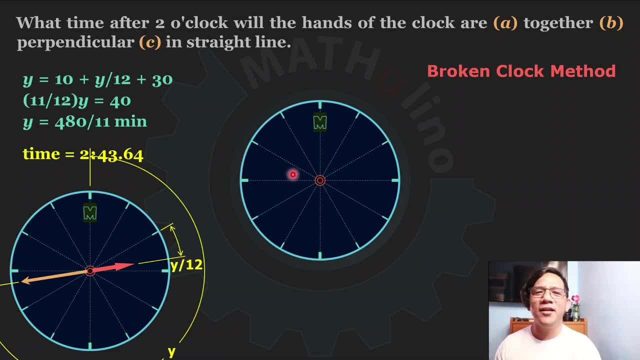 the this type of drawing. in fact you can. you can solve without the drawing. just imagine the move, the hands of the clock, which means that the hands of the clock, the the two o'clock mark is pointing at the top lock, that the hour hand is pointing at the top lock and this minute hand will point. opposite to the two o'clock. two o'clock mark, which means it will be in 2 o'clock, other hand will be 73.5, 40常 times 354. in that much time the hour hand will be pointing at the hour hand with internet. and now. 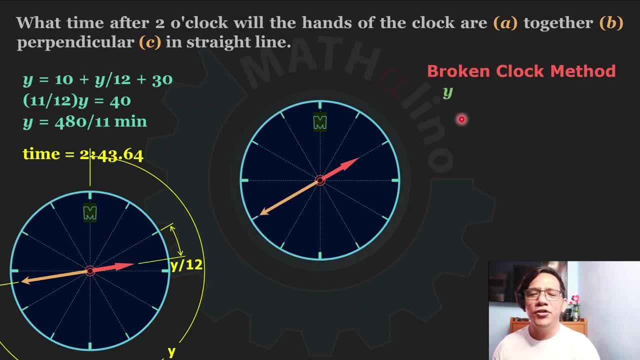 point to eight o'clock mark by using the hour marks. we are going to use the number 60 over 11 times 8.. that is the answer: 60 times 8 is 480 over 11.. okay, and using the angle, how? how many degrees? 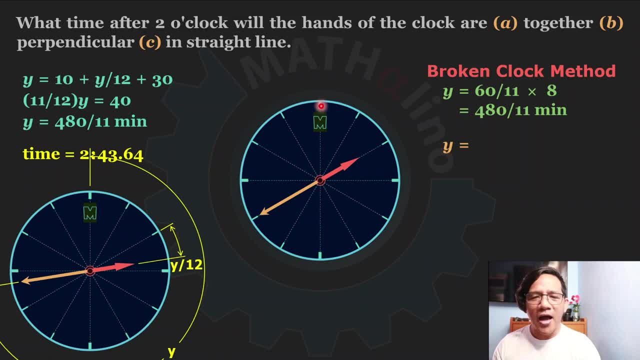 from from, uh, 12 o'clock mark to 8 o'clock mark. okay, that is 30 times one, two, three, four, five, six, seven, eight, thirty times eight, of course. thirty times eight, okay, two over eleven times 240 degrees, that is 30 times 8, 240.. that is the answer: 480 over 11.. chicken joy, baby. that's it. 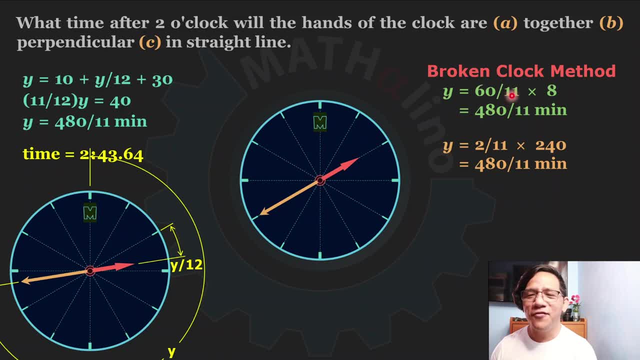 that's the shortcut solution: 60 over 11 times the hour mark, uh 2 over 11 times the number of angles. sir, i already encountered that approach, but it's only applicable to quadrangle angle, like like together, perpendicular straight line. i don't know, i don't know your source, but if that is your source meaning, 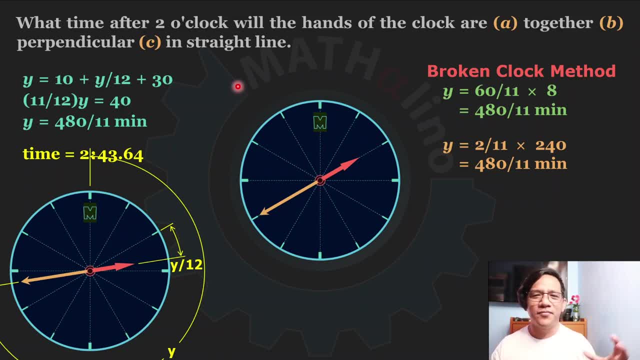 they did not get that. the concept, the full concept of the method. okay, maybe they are following the method blindly. if you have this method, don't just follow blindly. go, go for the core concept, okay. that's why, if you are going to study anything, and if you are going to study especially mathematics, go with the basics. 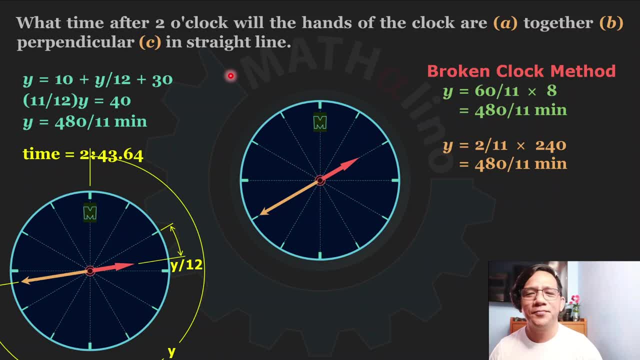 the basic concepts, because if you go with the basic uh, you can create or you can develop your own strategy in solving, in attacking any problem. right, that's the best method. okay, Now this is actually applicable to any angle, not just quadrantal angle. Let us say this problem: 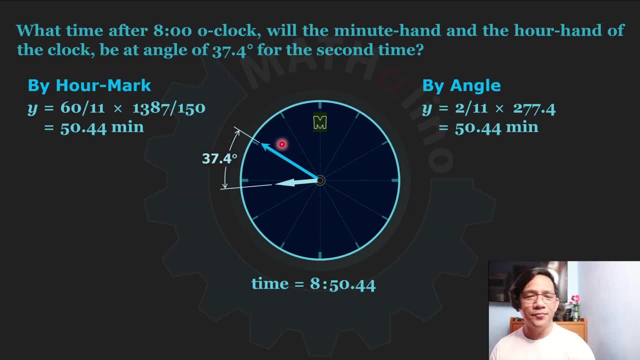 Let's go back to our number one problem: How to solve this one. Okay, This is 37.4 degrees By our mark. let us have this one: Y is equal to 16 over 11.. Of course, we are going to use the broken clock method, which means that this hour hand will remain at 8 o'clock mark. 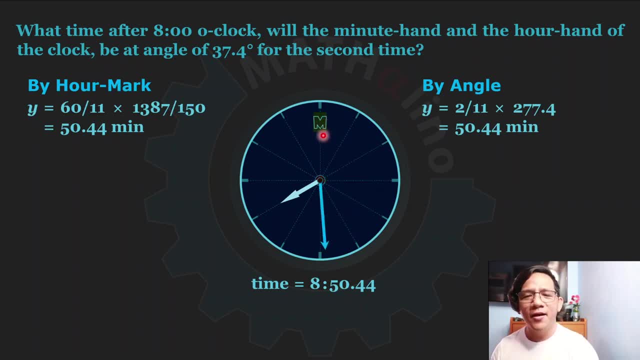 We are only going to move this minute hand The moment. the minute hand will subtend an angle of 37.4 degrees for the second time. that is the position where we are going to solve. Our hand is tucked at 8 o'clock. 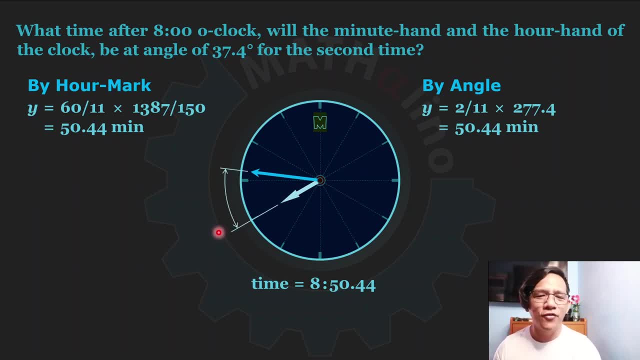 The broken clock method. Okay, This is the 37.4 degrees. So what is our Y? What is our Y? 60 over 11 times what. How to get this number? That number is actually the hour mark at this position. 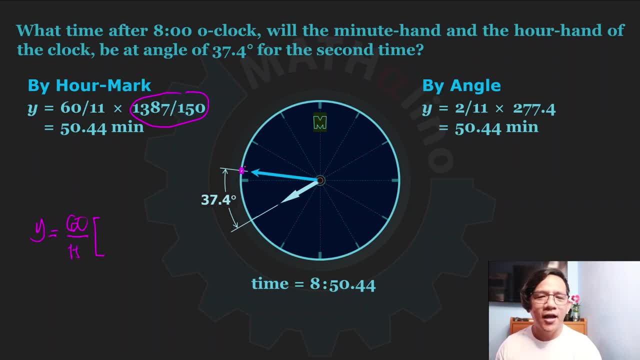 Okay, The hour mark at this position- How to do that? That is 8.. The hour marker is 8 plus 37.4.. But take note that 37.4 is angle, not an hour mark, So we are going to convert that into hour mark. 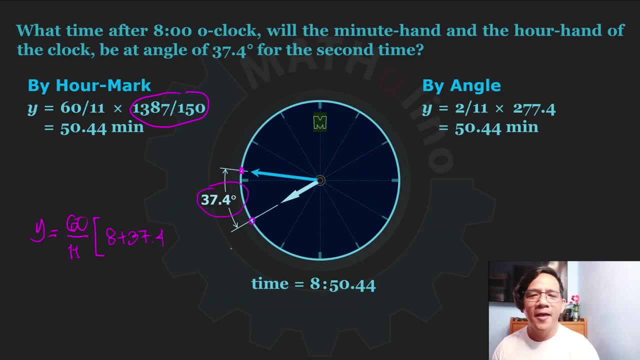 How to convert this into unit hour. Okay, Note that every hour 30 degrees, which means we are going to divide this one. Okay, 37.4 by 30.. That's the number. That's the answer, Boom. 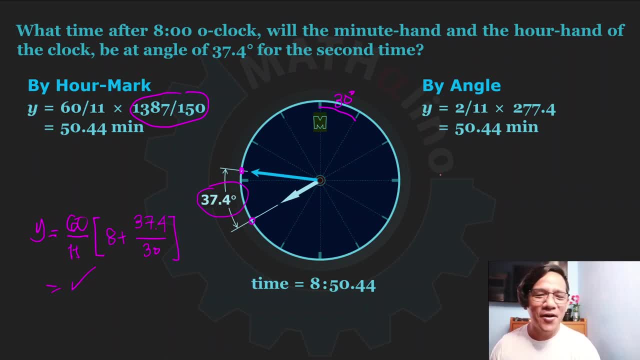 You're done. That's it. How about by angle? So, by angle, we are going to use the number 2 over 11.. Okay, Then we are going to write the angle here From this 12 o'clock mark. 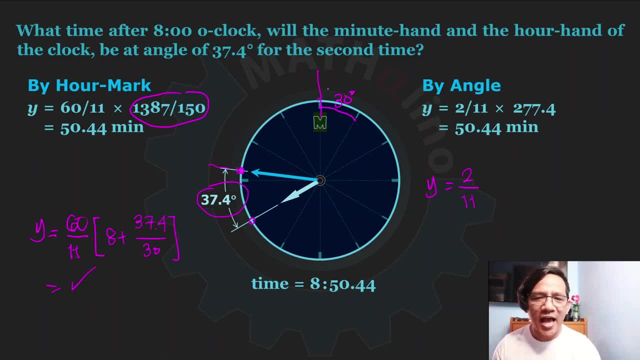 Up to this point. Up to that point, What is the angle? Let me write it in another color. I use yellow. Okay, From 12 o'clock mark up to this point, we need to find this angle. Okay, That angle actually is. 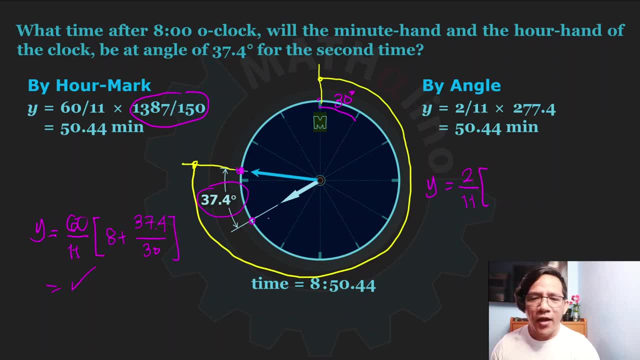 First we have this: 80.. It's zero. What's this angle? Eight times 30.. Okay, Eight times 30.. Plus, Okay, Eight times 30.. What's that? Eight times 30. Okay, Plus. 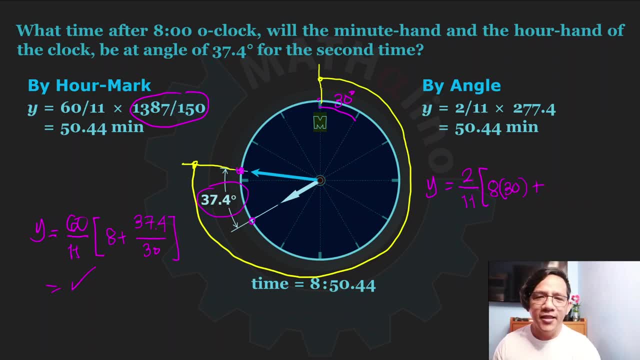 Okay, Okay. Next is the value. Ok, Now we will add down here. We are going to add down here, Ok, Ok, Let's start with this angle. Okay, One, two, three. That's in here here. 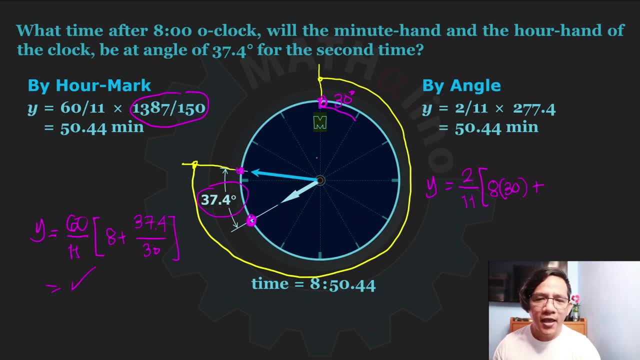 What do we have here Here, Here? Here is the angle. So we are going to subscribe this. Let's add this: Look, Look, Look Here Here. Ok, Then let's give this angle here. Okay, 8 times 30, that's the 8 times 30 degrees. okay, plus 37.4, that's the 277.4 degrees. 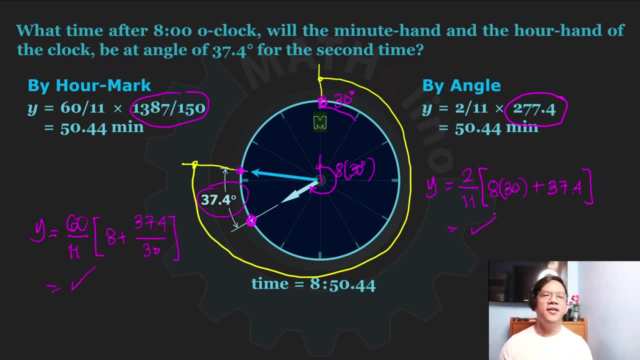 and that is the answer. where do you see any time? you can do that. any relationship between the angles, not confined by quadrantal angles, okay, any angle will do Next. now, the purpose of this video actually is for us to understand what happened. where. 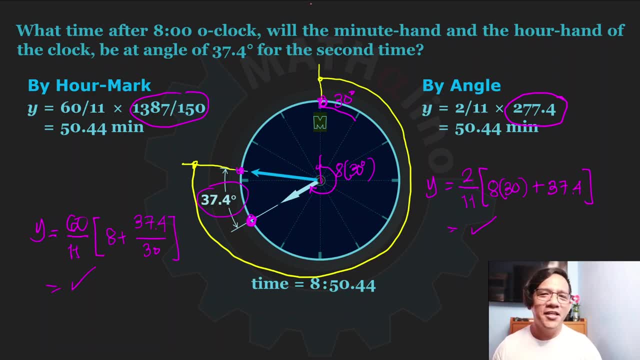 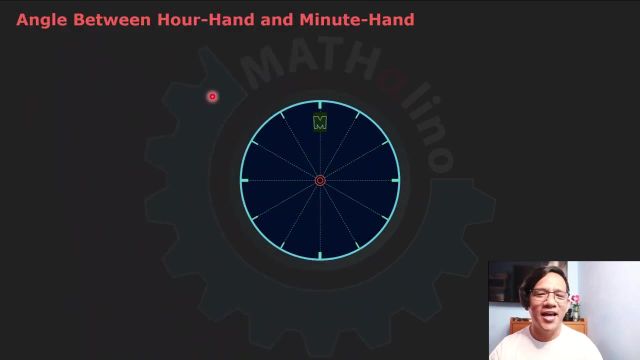 this formula came from this: 60 over 11, our shortcut, or 2 over 11, either of the two will do. okay. Let's go back to the very basic. let us generalize our discussion. let us say that the minute 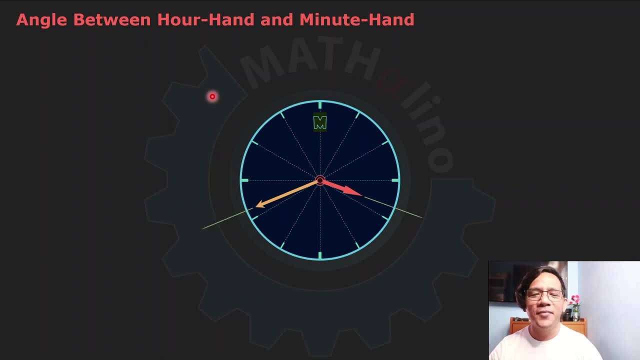 hand and the hour hand of the clock subtend an angle of x degrees. okay, You can use theta if you want to. I just use x for this discussion. okay, But take note that x is an angle. that's why it is convenient if you are going to use yourself. 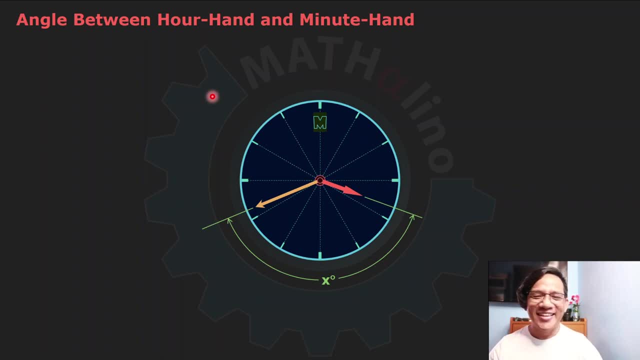 theta. okay, So what time is it? Let us call that in this case 3, 3y. okay, This is our y, from the 12 o'clock mark to the minute hand y and, of course, from the 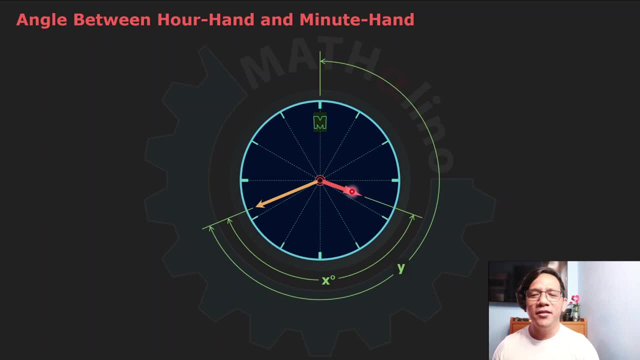 3 o'clock mark to the hour hand. the movement of the hour hand is actually this one, which is equal to y over 12, and from here to here we are going to use the 3 o'clock mark to the hour mark. this is our hour mark. it happened that we are at 3 o'clock, so what is the value? 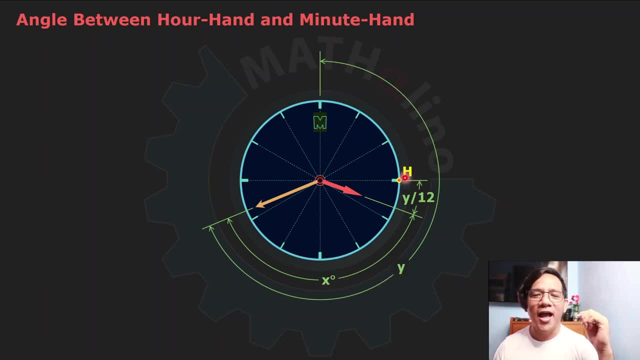 of y in terms of x and h. the hour hand? I don't know, this is not the hour hand. this is the hour mark. okay, From the figure we can write, y is equal to what? From here to here? that is hour mark, but of course our equation is in minutes. according. 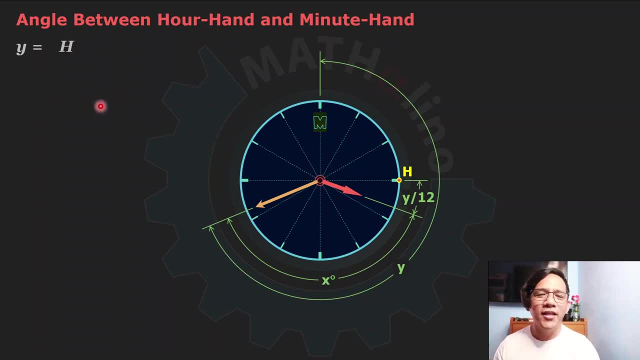 to our discussion earlier. in this video We are going to write our equation in unit of time, minutes. so how many minutes? from here to here, Every hour marks 5 minutes, 5 minutes, 5 minutes. a total of 15 minutes. this is actually number. 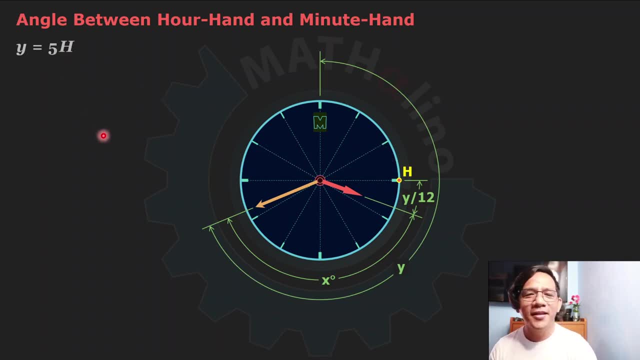 of the hour marks times 5, okay, Plus y over 12, where this 5 came from. This is conversion from hour mark to minutes. I will repeat: 5 minutes times plus 5 minutes, a total of 5 times h minutes. our h here is 3, okay. 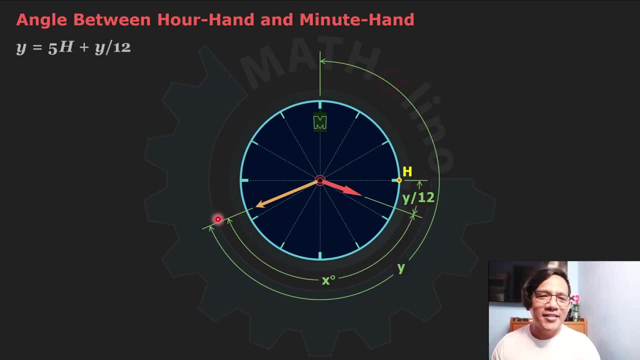 Plus y over 12, plus angle x. take note that this x is not compatible with the minutes of 9, we are going to convert this into minutes. what is the conversion? Very easy. we know that. we know that. where is my laser pointer and my pen? we know that. 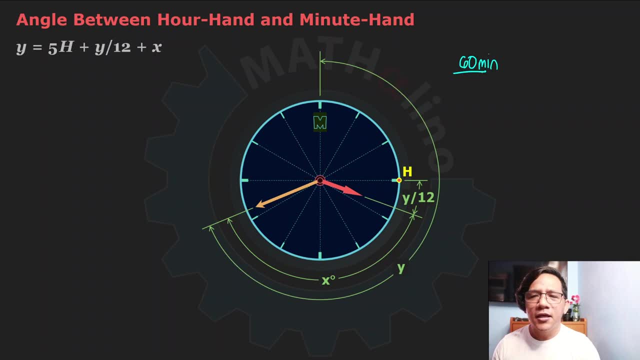 minutes is equivalent to 360 degrees. one revolution, okay. 60 minutes of time, 360 degrees angle. this is also equal to: if you want 15 minutes of time, 90 degrees of angle, okay, and this is one out of six and that is the conversion. so we are going to divide this x. 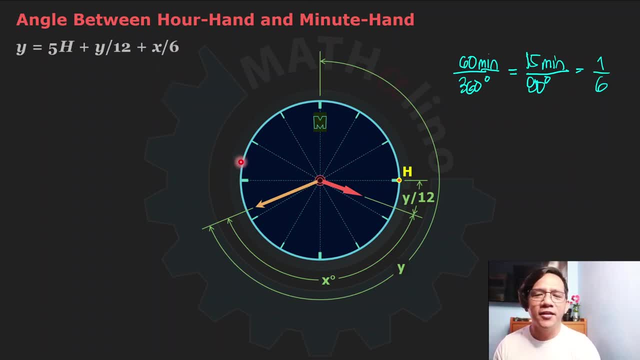 by six to convert degree into minutes. now all our units here are compatible. this is in minutes, this is in. this is an hour, but multiplied by five it will become minute. of course this is also minutes and this is also minutes already, because we divide it by six. 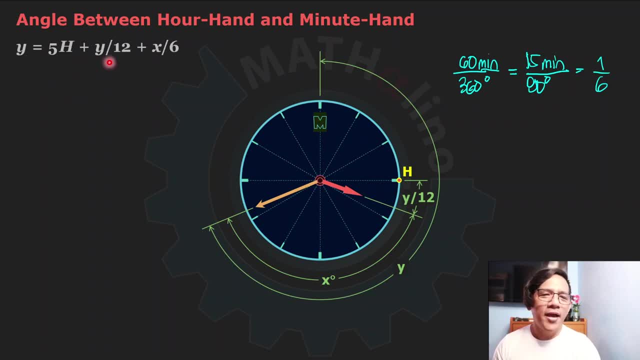 okay, we can proceed. 1 minus 1 over 12, that will become 11 over 12. of y plus is equal to 5h plus x over 6. divide both sides of the equation by 11 over 12, we have this: y is equal to 5 divided by 11 over 12. that will be 60 over 11. 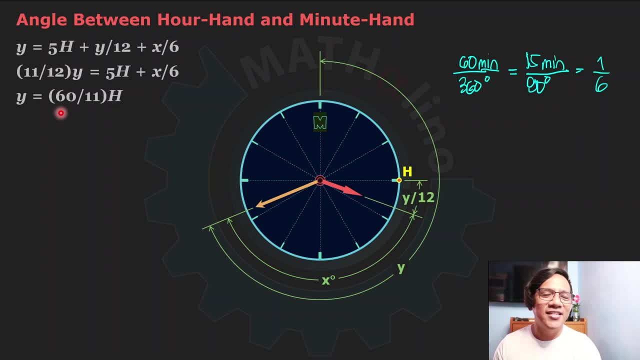 that is the this. uh, where that 60 over 11 came from? it came from here: 60 over 11 of the hour marks plus 11 over 12, 12. okay, 11 over 12 as 1: 6. i mean 1, 6 divided by 11 over 12. that will become 2 over 11. 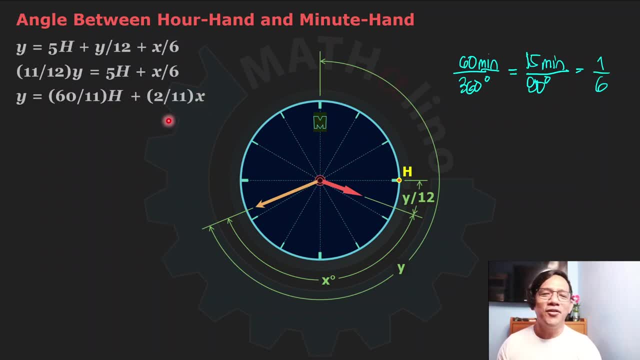 times the angle in degrees, where the 2 over 11 came from. it came from here. okay, from this equation twin, 60 over 11 and 2 over 11 times the hour marks times the angle. you see that now there are instances that our angle or our- excuse me, our minute hand is uh, will not pass. 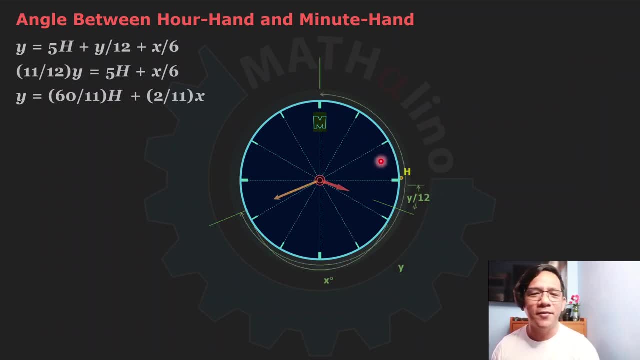 through the our hand. yet what i mean is this one, the position of the minute hand, and our hand is this one. where are you? okay? and this is the x degrees, which means that the minute hand is still at the back of the our hand. if we are going to, if we are going to. 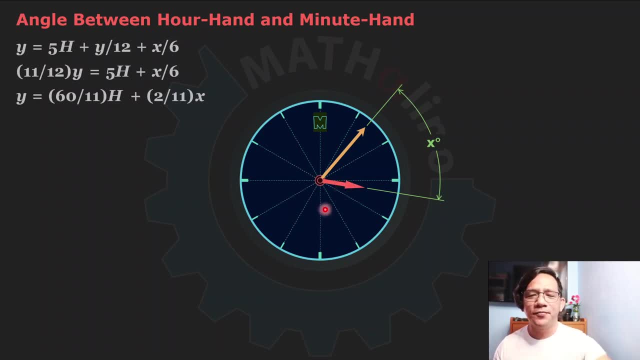 so say, front for the movement that is clockwise. of course this is a clock, the clockwise movement in the clockwise direction. we call that the front, and at the back and in. if we go counterclockwise, that is at the back. okay, so our minute hand is at the back of the, of the 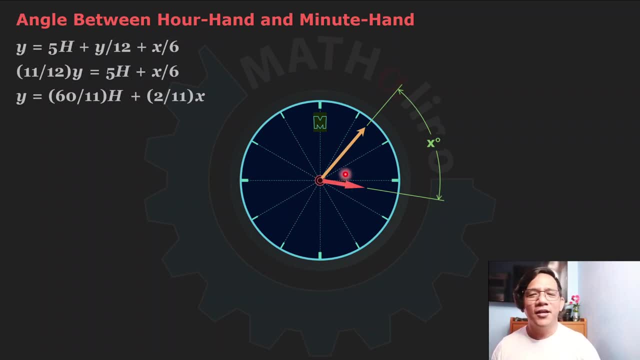 of the our hand in this position. what is this time? let us call this again 3y. okay, this and this number of minutes here is y by minutes. what is the value of y? of course, this movement of the hour hand is y over 12. okay, that is y over 12. let us write the equation for the value of y. we have this y. 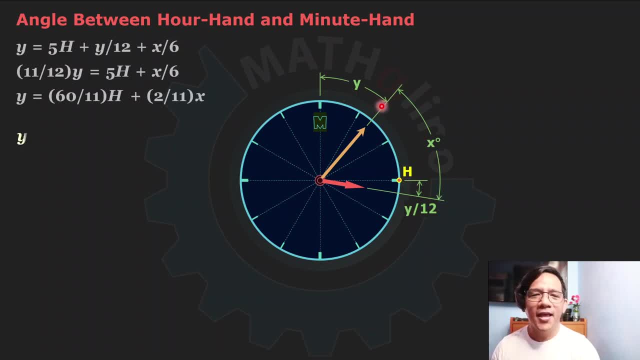 and this is the hour mark: y, okay, plus x degrees. of course, we are going to convert this into minutes. how to do that? divide it by 6, okay. this is going to be h here, divided by 6. okay, if you cannot see what the syntax is, of course. 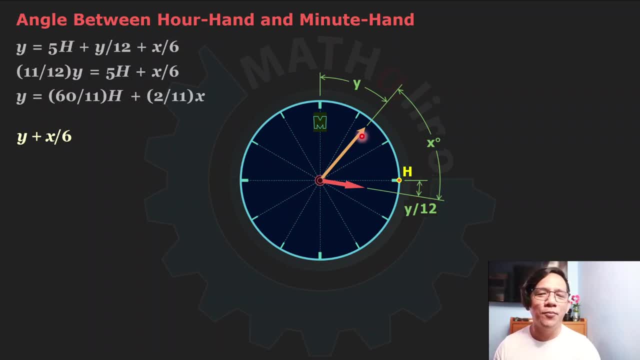 cannot memorize that that over six. just do the proportion: 15 minutes, 90 degrees all over 90. this is 15 over 90. or that proportion, uh, 60 minutes all over 360 degrees. okay, to convert that, that is also one over six. they're also one over six. yeah, this one is equal to y plus x degrees. 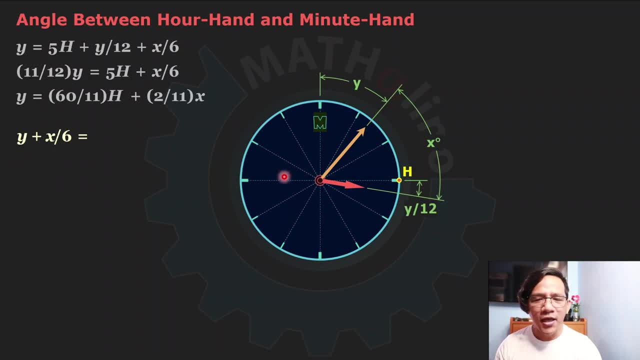 we. that is the equation we came from. from 12 o'clock mark up to this point. that is the y plus x over 6 from this mark up to this point. okay, that is also equal to the hour mark: 5, 10, 15. okay, the hour mark, which is 3 here times 5 to convert that into minutes plus y over 12. okay, 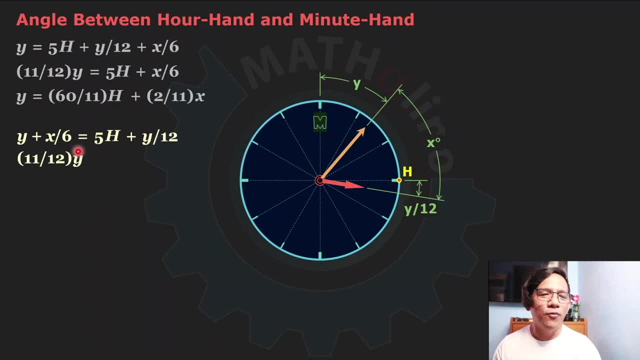 1 minus y of 1 over 12 is 11 over 12 of y, then 5 h minus x over 6. transpose this one then divide 11 over 12, both sides, we have this. y is equal to 60 over 11 again of h, and this one is: 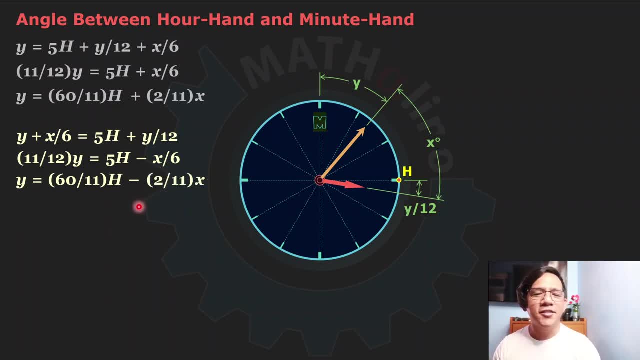 minus 2 over 11, again of x. okay, that is our equation. if you observe that equation into, compare this equation into here, we only have the difference of the angle. okay, so we can write our equation this way: 60 over uh, plus or minus for 2 over 11 of x. 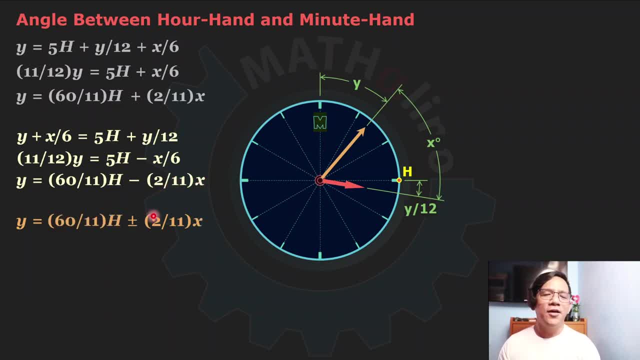 plus 60 over 11 of h. now this plus or minus arc actually only represents the, the position of the minute hand with respect to the our hand. positive if the if the minute hand is at the front of the our hand. negative if the minute hand is at. 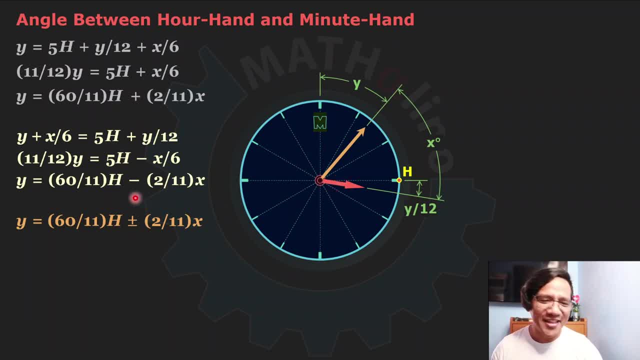 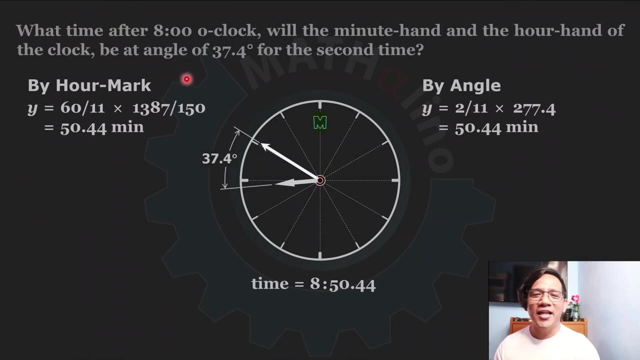 the back of the hour hand. that's it. that is our equation. let us tie this with our problem. okay, how to use this equation. let's say, for from our problem using that whole equation, let me write that whole equation pen. okay, our equation is 60 over 11 of. 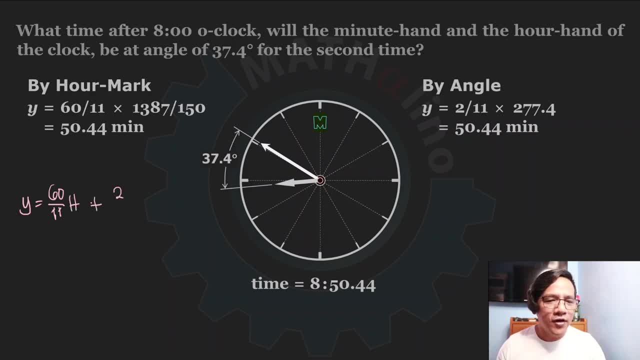 plus 12th of 12, nf of the hour, march, plus 2 over plus or minus, plus 2 over 11 of the angle. okay, of the angle. so we have this one, the number of ours. this we are. we are going to solve this way this, this, uh, value. this is the y from the twelve O'clock mark. 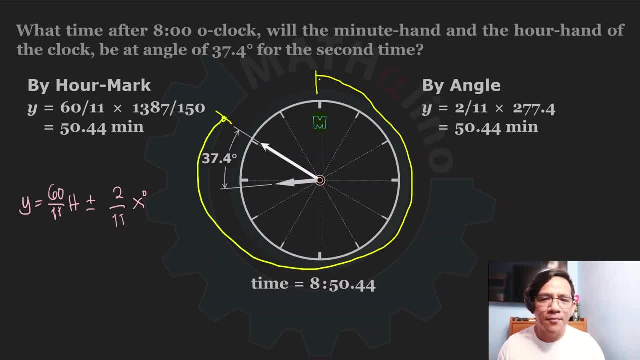 to the mini 10. this is the actual position. this is not the broken clock method, actually the the equivalent to that. drawing in our figure in in our previous solution, the, the concept based solution. okay, we have this. y is equal to 60 over 11 of the hour mark. of course we. 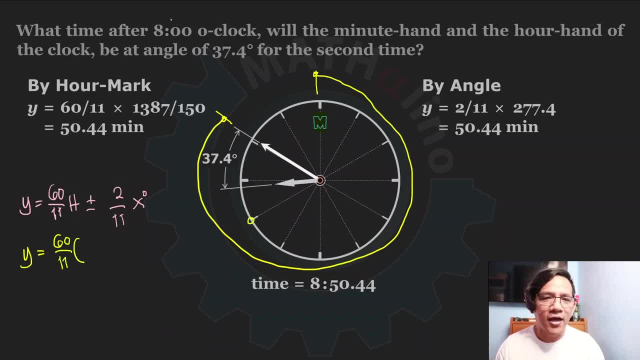 are going to use the hour mark of the, the eight o'clock. okay, for the base hour mark eight o'clock plus two over eleven of the final position, angle: 37.4. that is the answer. okay, 50.44, you can do that, i will not check it here. 50.44, that's it. that's how to use that problem. but but, sir, uh, when we 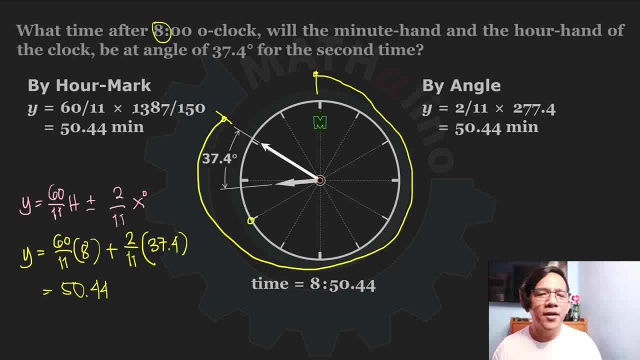 solve this, this uh problem earlier. you just use directly. use this one i. you just use directly. use this one i. either 60 over 11 only, or 2 over 11 only, not both. why is that so? okay, let us understand this equation. let's understand this equation. 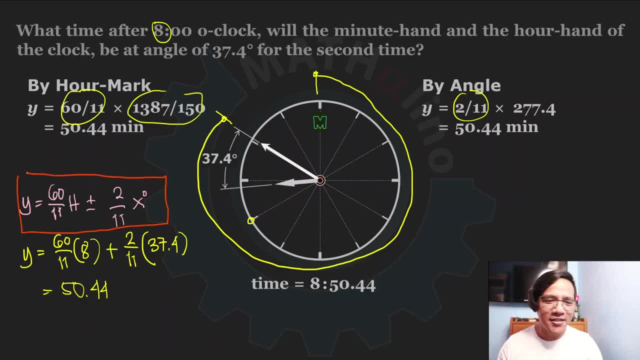 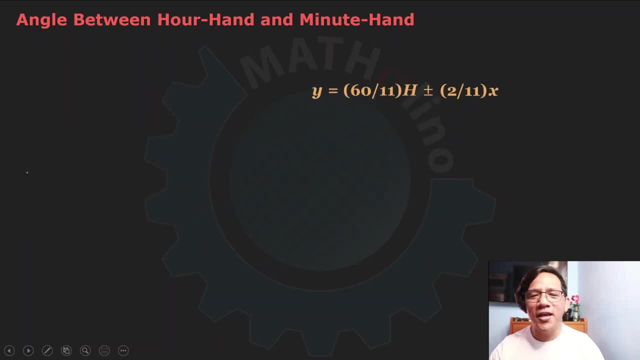 the idea is to understand fully this equation. let us discuss that. of course, it will help us if we have an example. okay, this equation, actually, let's have this example. there is my example, this one, this: this equation actually is, uh, linear in x. that's why i use 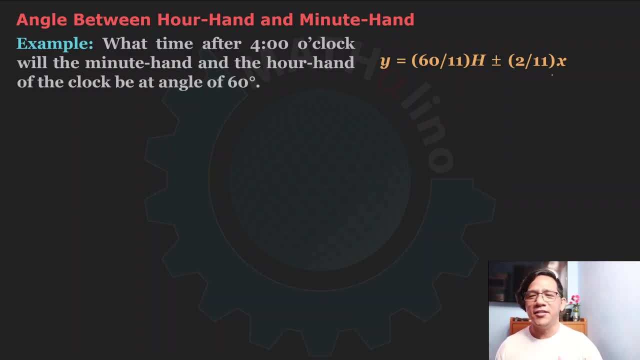 x here instead of theta, so that it is very easy to see that this is linear in x straight line. this is in the form: y is equal to mx, mx plus b. okay, which means that this quantity, this quantity, is actually the y intercept in the xy plane. 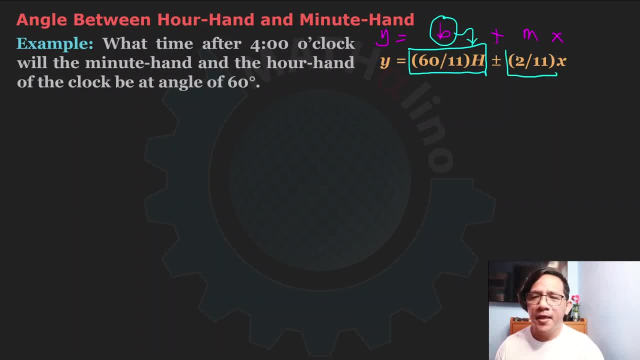 y intercept, and this quantity is the slope of our line. okay, take note that our slope here is positive. we are going to use positive slope because this plus or minus this represents only the position of the hour hand with resp of the minute hand with respect to the hour hand. 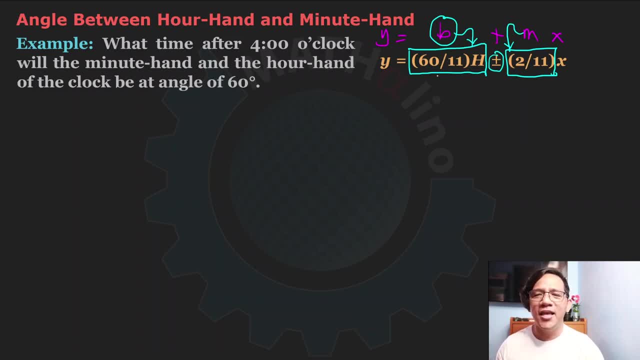 so we can plot this graph straight line in the xy plane. okay, let us plot this, this equation, in the xy plane. we have this: uh y intercept 60 over 11. we have this problem. what time after four o'clock will the minute hand and the hour hand of the clock be at angle of 60? 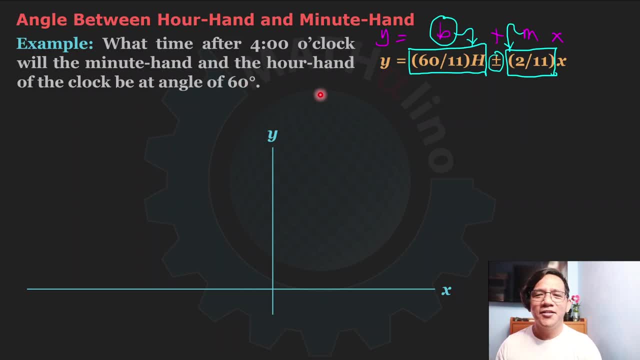 degrees. okay, that is the question. so we are going to start at at the y intercept. the y intercept is 60 degrees over 11 of h. if you are going to use, h is equal to 4. okay, that is 21.82. let me write it here. we have 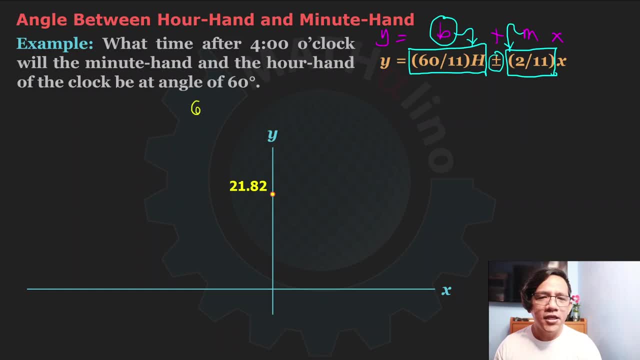 this 21, uh 60 over 11 times 4, that is 21.82, and we have a line that will pass through this y intercept, a straight line with the slope 2 over 11.. so meaning this is our line, okay, a positive and upward line. the slope is positive: 2 over 11 y. 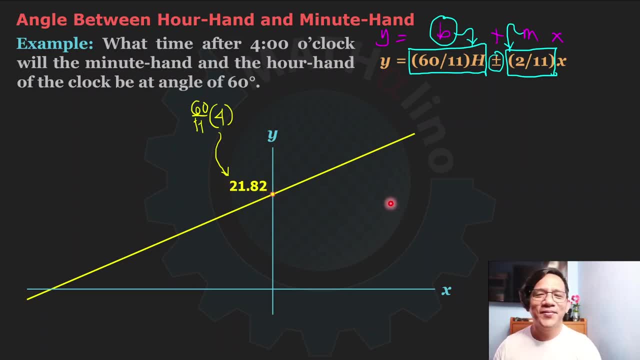 intercept 21.82. okay, now the question is, what time? after four o'clock, that, excuse me that this, uh, The angle of the clock, The hands of the clock, Will subtend 60 degrees angle. Let's do that, Let's move this Equation, Erase the writings. 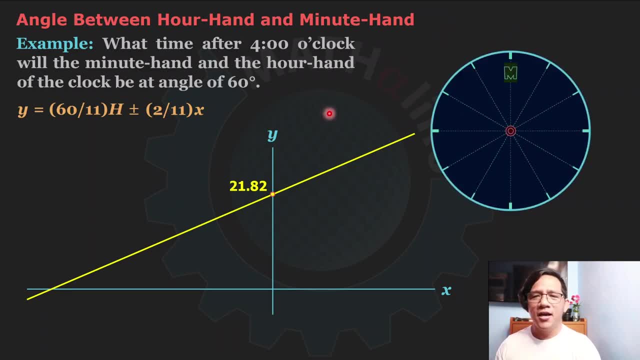 And let us illustrate using the The. What is that? The position of the hour hand, The final position. This is not the broken clock method. This is the actual movement Of the minute hand and the hour hand. This is the 60 degrees For the first time. That is, the 60 degrees for the first time. 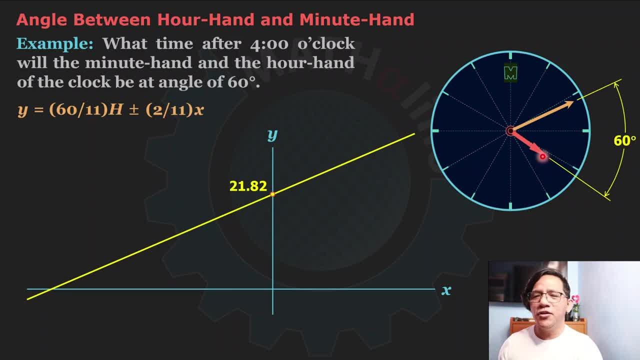 What time is it? Because in this position, The hour hand is behind The minute hand. The minute hand is behind The hour hand. The minute hand is at the back of the hour hand. We are going to use negative To solve for the value of y, Which means that 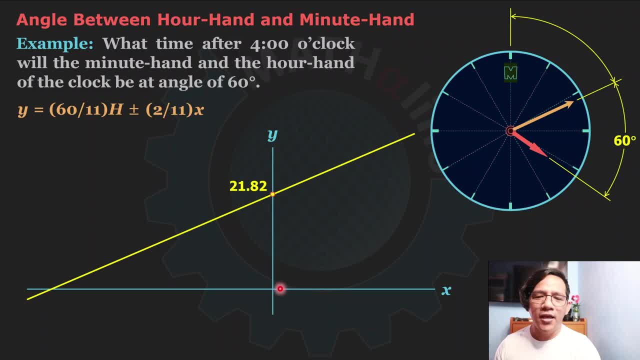 Our angle 60 Is actually To the left of the origin. So to solve for the y1, This is our angle 60. Negative 60. That's the purpose of Plus or minus Negative 60. Now, what is the ordinate Of this line at x Is equal to negative 60. 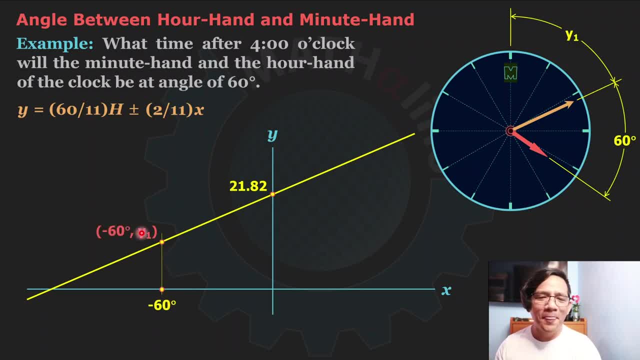 What is y1?? You can use this equation. Okay, The equation of this line Is 60 over 11 of h. Our h is 4. That's it Minus. When we say minus, We are going to drop By this amount. This is actually 2 over 11 of x. 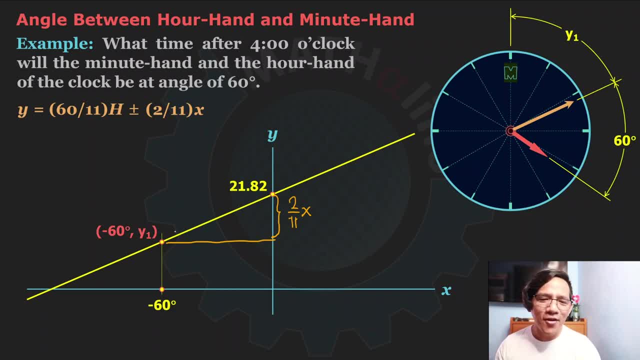 Okay, That is the value of y: 21.82. This is the 21.82. This value here, 21.82 Minus 2 over 11 of x. Okay, Let's erase that one. Replace this by 9. Okay, This portion here is 2 over 11 of x. 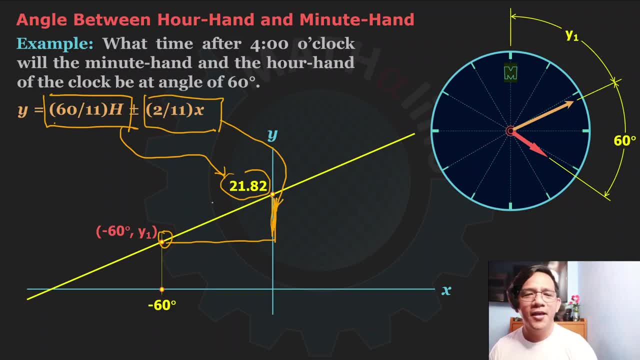 You drop by 2 over 11 of x. Actually, that 2 over 11, You can appreciate that With y is equal to The slope. The slope is rise over run, Rise over run, Which means that We solve for the rise. Okay, The rise is actually The slope. 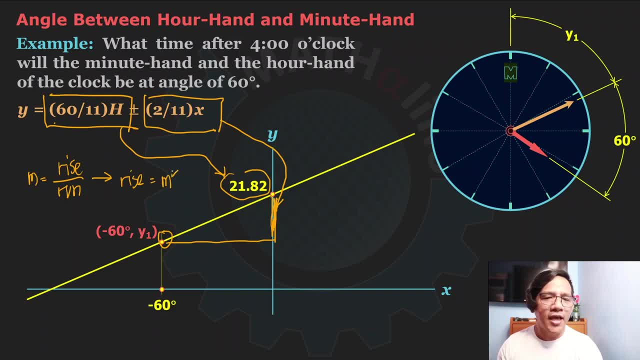 The slope is actually The slope Times The run. Okay, This is the run. It's equal to 60. Okay, That's why, To find this height, To find this height, We have this slope 2 over 11 Times the run: 60, 21.82 Minus the. 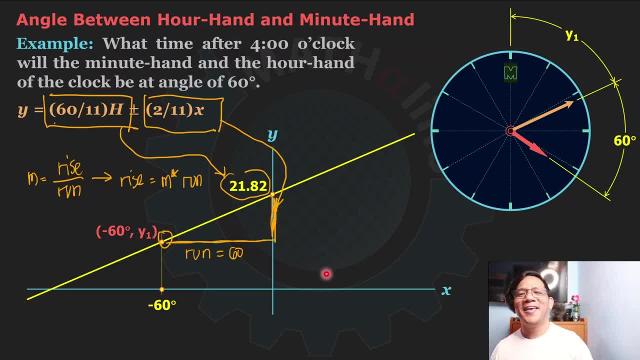 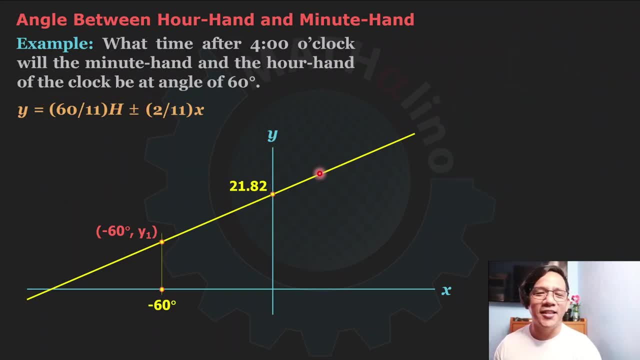 The rise, That is the y1. You see that. How about, For the second time, 60 degrees for the second time. Okay, Let us erase that writings. We have this Position of the hour hand and minute hand To some 1060 degrees angle For the second time. 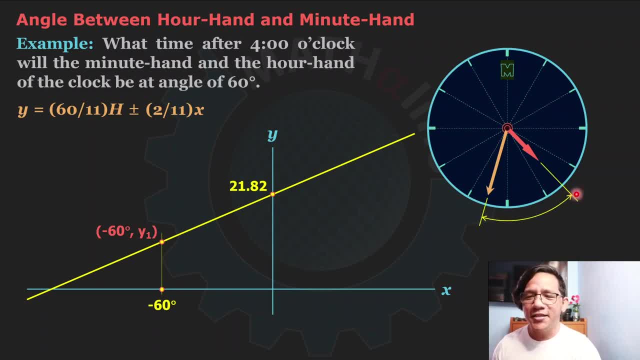 That's it. What time is it? This is the 60 degrees, Okay, And this is the angle. Okay, Let me check if For the video feed. All right, Let's continue. Our minute hand now is At the front of the hour hand, Which means that we are going to use. 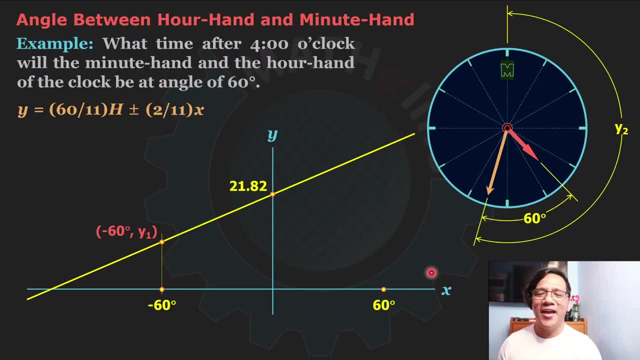 Positive 60 degrees. Okay, Our x is angle, Our x is angle Positive 60 degrees. The question here is: What is the value of y2?? So we are going to project the 60 degrees To the line, And what is the Ordinate of this line? 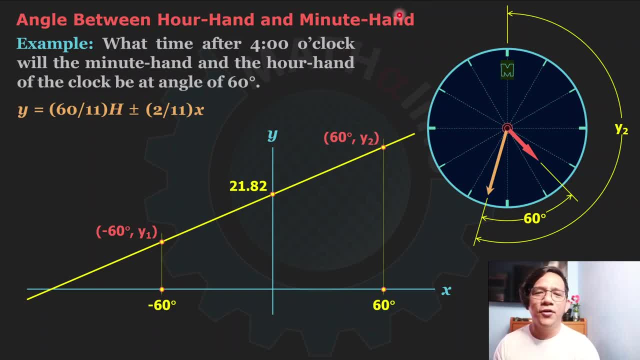 We call that y2. Now, to do that, Of course, We are going to add 21.82, Which is this one. Okay, This one. Let me change color. Uh huh, May use This color. It's dark Orange. This, The same color. This 60 over 11 of x. 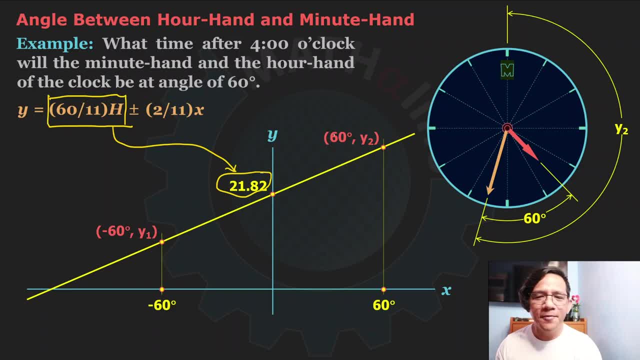 Is this one again, Of course, we mentioned it earlier. And This 2 over 11 of x Is actually this vertical distance here, Vertical distance. Okay, This vertical distance is 2 over 11 Of x, Where x is the run. Okay, X is equal to the run. 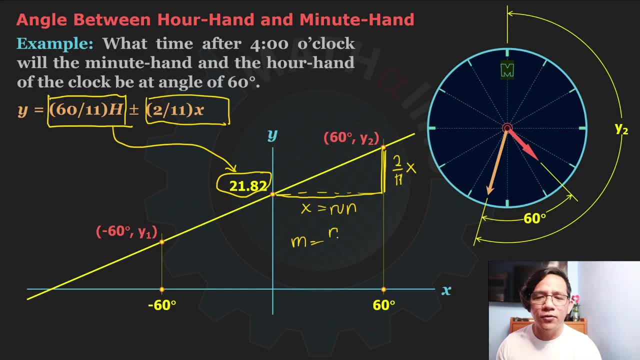 From the equation: Slope is equal to rise Over run, And our slope here is 2 over 11. That's it. That's how we interpret that equation. How about, sir, For the solution With using 60 over 11 alone, No 2 over 11 of x. 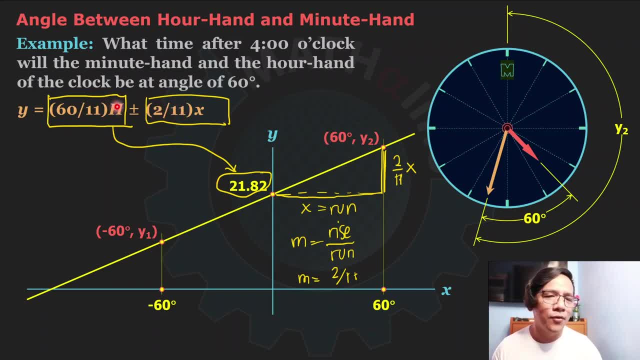 Or the 2 over 11 alone, With Without using the 60 over 11 of h. How to do that? The answer is: Translation of axis. We are going to translate the axis Instead of Making our origin at here. We are going to translate this point. 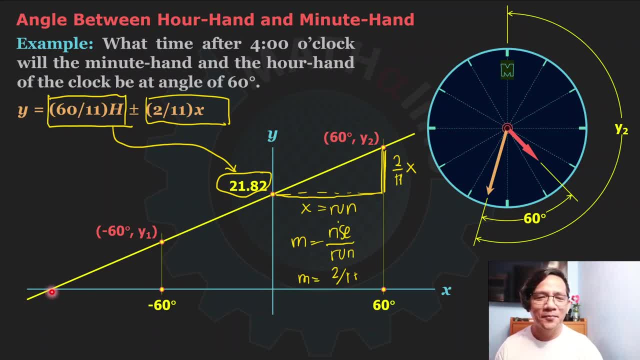 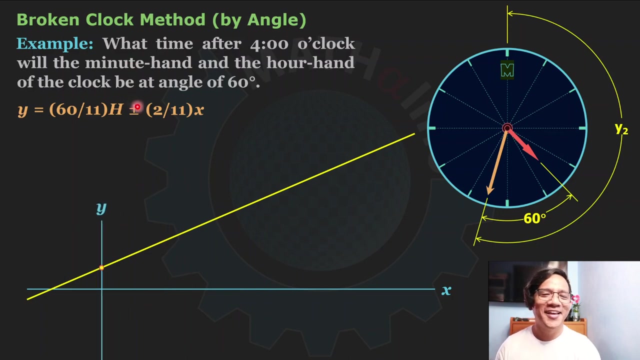 To the X intercept. Okay, To eliminate the other. This h, This value of h. Let's do that. Okay, This point, We are going to translate it here. Now, that is the broken clock method concept. That is actually translation of axis. Okay, This is now our origin. Okay, Take note that this origin 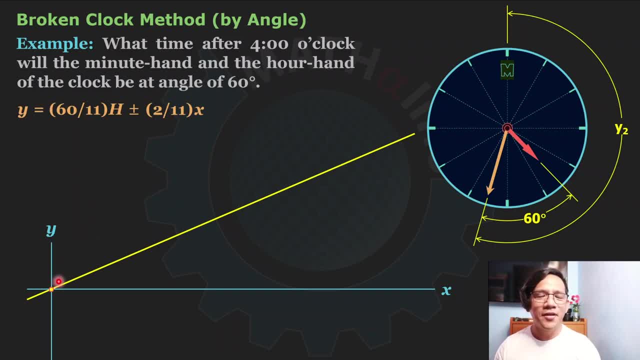 From the original equation: This is the x intercept. What we did, is We just? We just put this h into 0. We push that into The x axis. Okay, That's why this is not included in the solution. You get that Now. We are not going to concern ourselves here. 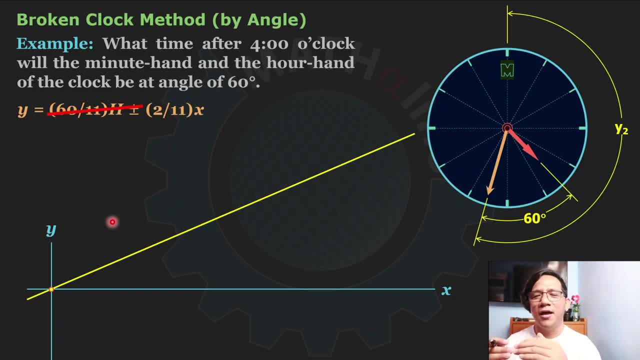 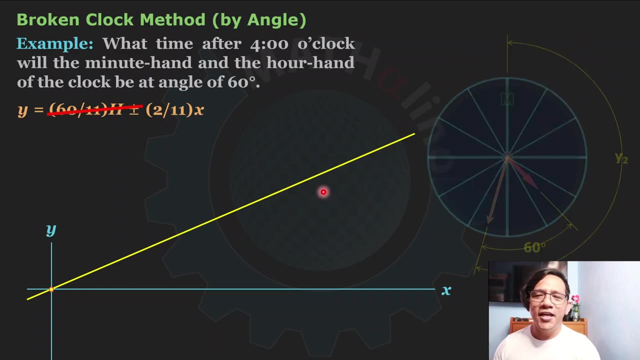 Ourselves here in. If the minute hand is at the back of the hour hand Or it is at the front of the hour hand Doesn't matter anymore, because Everything here is to the right of this point. This graph So meaning For 60 degrees for the first time. 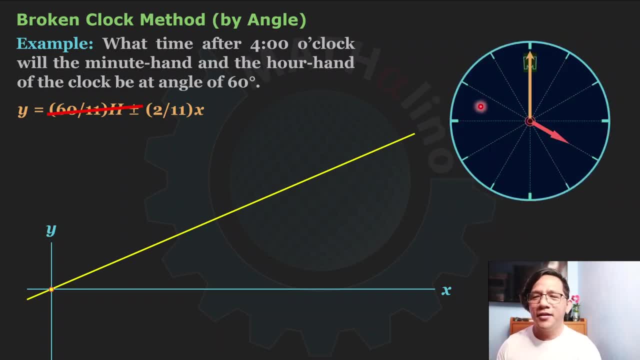 Broken clock method. Okay, This will not move 60 degrees. for the first time It will go to the 2 o'clock mark, Which means by By angle. This is 60 degrees. So from here Forward with 60 degrees, Okay. The question is: What is the value of y? 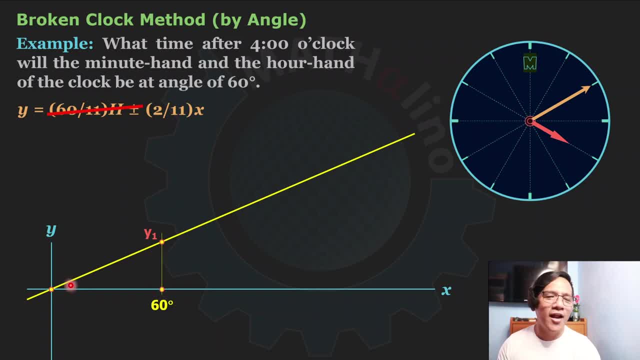 We call that y1, Y1, Rise over run. That's it. Y1 actually is Rise over run. This is equal to Slope is rise over run. Let me write it Again: Rise over run. The rise is Slope Times The run. The run is 60. 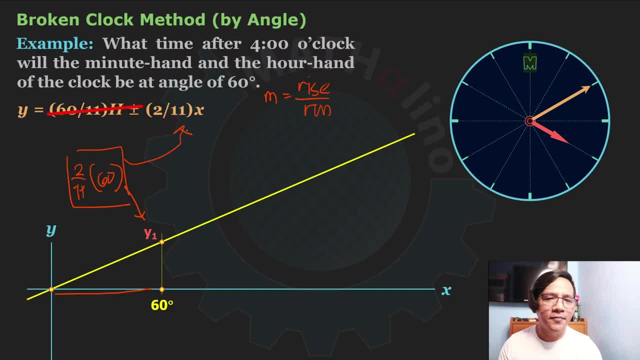 That's it: 2 over 11 times 60. The x: Okay, How about 60 degrees for the second time? Okay, This is 60 degrees. 30, 30- Okay, For the second time, We move actually from 12 o'clock mark To 6 o'clock mark. 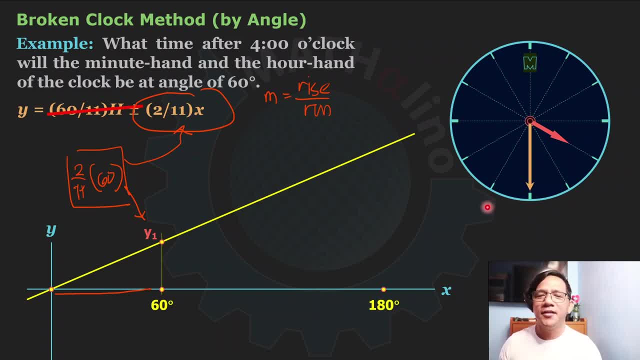 A total of 180 degrees. Take note that. Take note that x From here is When we use the, When we use the, When we use the broken clock method, Our reference point becomes the, The This 12 o'clock mark In non Non broken clock method. Our reference point is the. 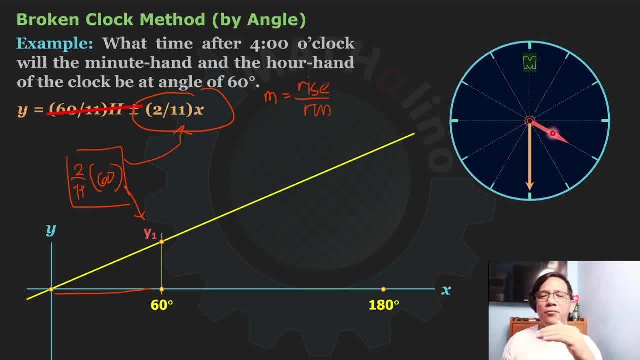 The. The Initial point of the hour hand. Initial position of the hour hand. Okay, So this will become 180 degrees. What is that? y2?? By rise over run, We have this 180 times, 180 times 2 over 11. That is the answer, Okay. 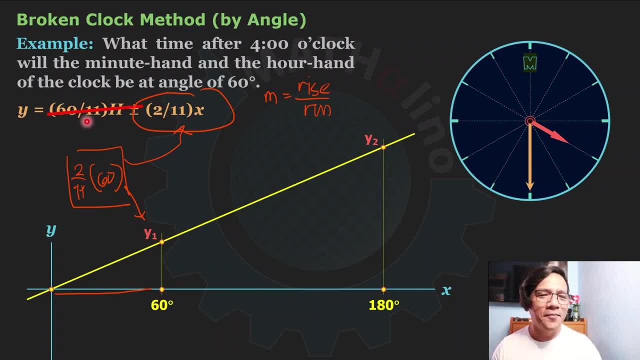 Very easy, Sir. how about the other one, That's 60 over 11? Of course, That is also a straight line. We are going to Consider 2 over 11 as constant And 60 over an h as the variable. Which means Which? Which means that we are going to replace x with h. 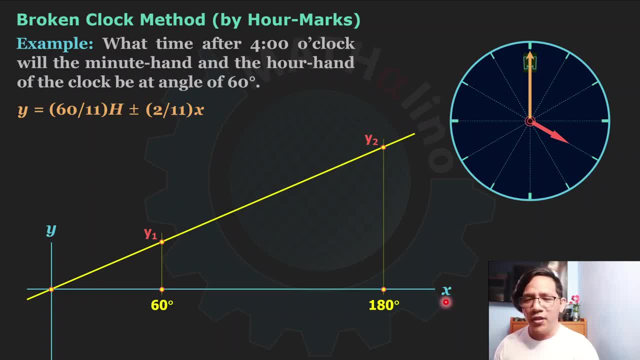 If We have the same line, Replace x with h, Like that one. What is y1?? The x is no longer included in the equation. Okay, So For the value of, For the value of y, We have this At At a time When the minute hand will subtend an angle.